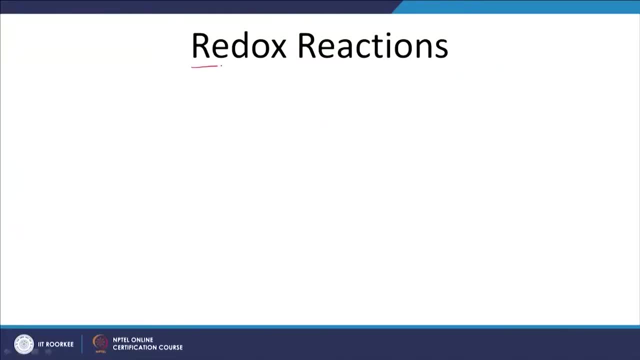 So let us look at what they are here. So obviously we have redox reactions. redox, obviously, what are we talking about? We are talking about oxidation and reduction reactions. So whenever someone refers to redox reactions, we are in the more or less obviously talking. 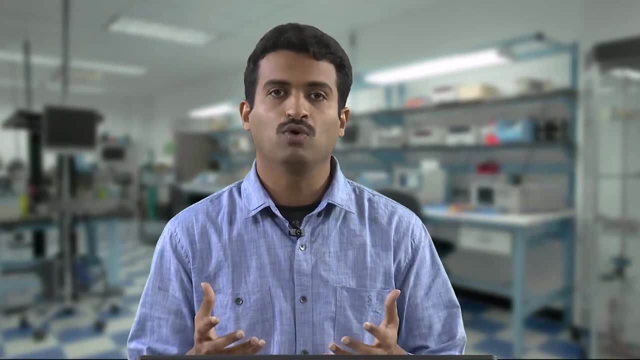 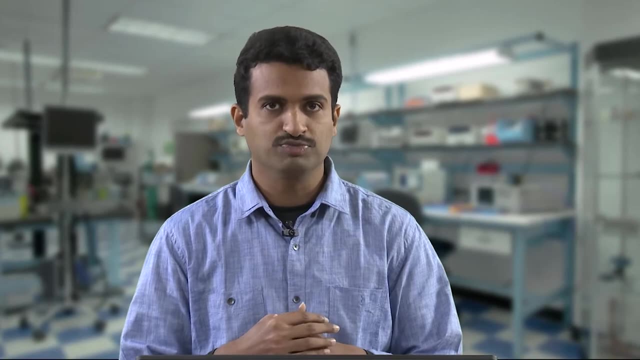 about oxidation and reduction reactions Which involve the transfer of electrons from one compound to the other. well, it is transfer, or it is going to be sharing, strictly speaking, but we are going to talk about that in relevant detail in the next couple of sessions, I guess. 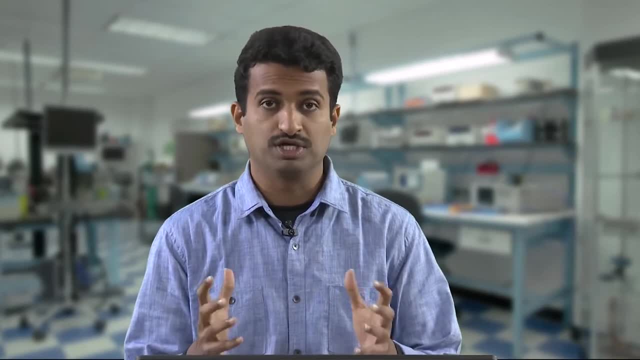 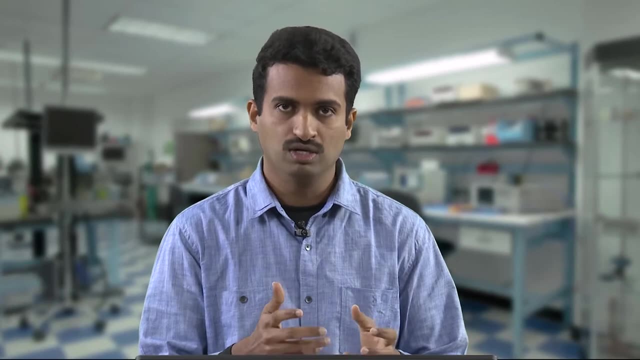 So here we are talking about electron transfer here with respect to redox reaction. So obviously, if there is an electron transfer from one compound to the other, the oxidation state of the relevant compound is going to change, or the relevant element is going to, or the atom is going to change. 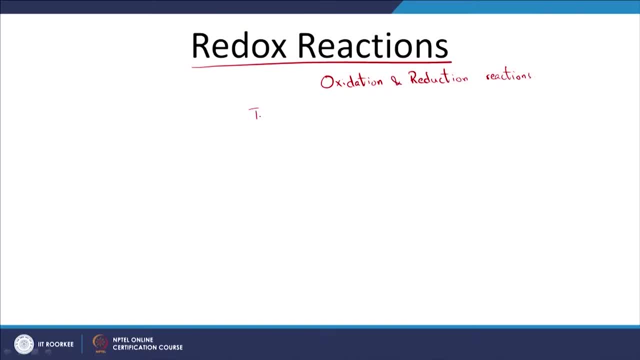 So again here we are going to look at some of the terms and obviously you know we have oxidation and reduction, So we are going to look at what oxidation is about, right? So this is the process of donating an electron, right process of donating an electron, and 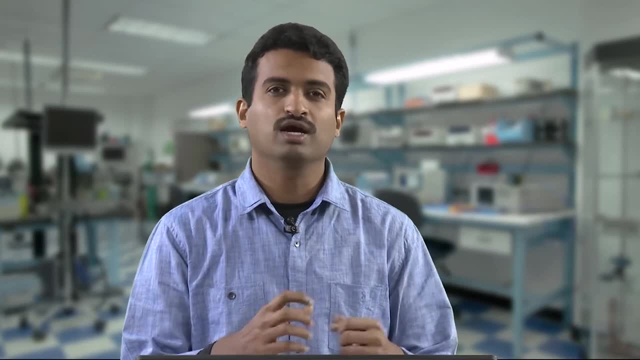 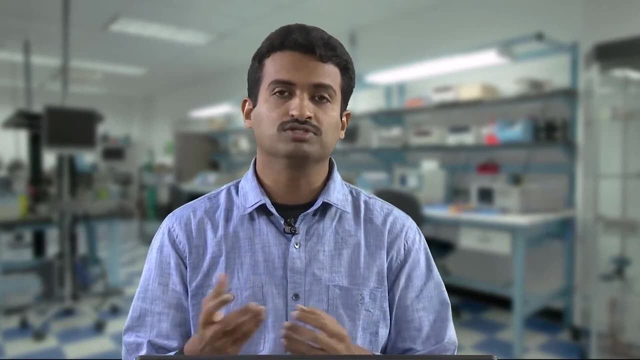 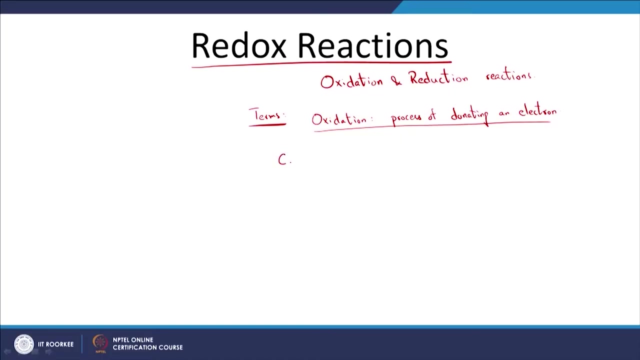 again, we see this widely. We are going to look at it in conjunction with reduction later on. but keep in mind that when we obviously talk about oxidation, it means there is a process of, for, you know, it is leading to donating an electron right. So we are going to look at an example, I guess, of oxidation that we briefly considered in. 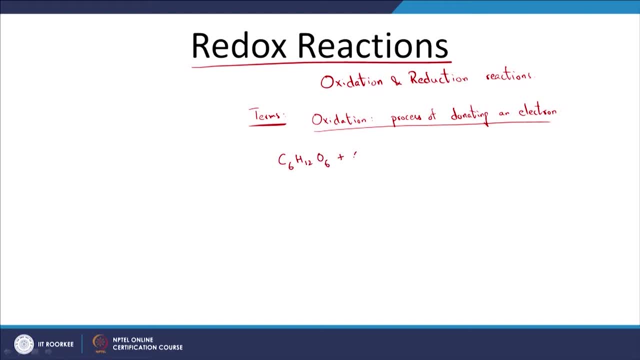 one of our initial classes- right And glucose and thus process, let us say, is 6CO2. so we are now donating the relevant electrons, right charge balance, you are going to have H+ And here this release of electrons that we see here in this point of reaction. with respect, 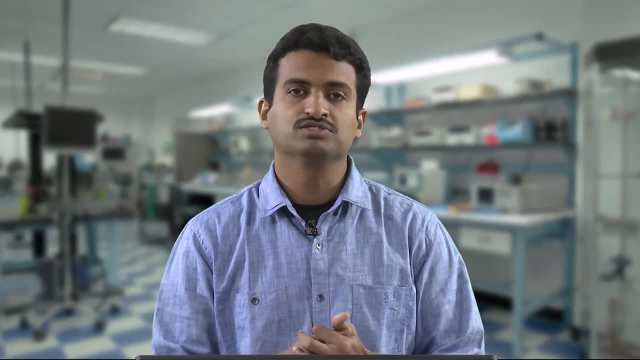 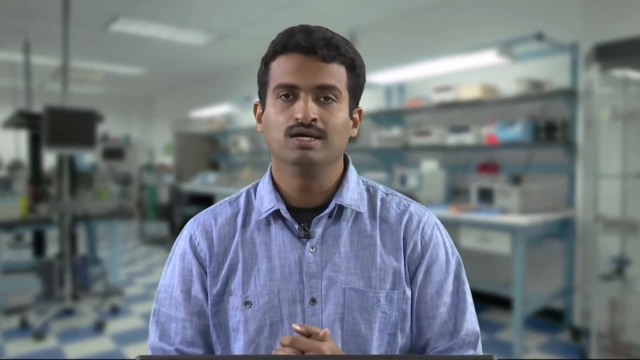 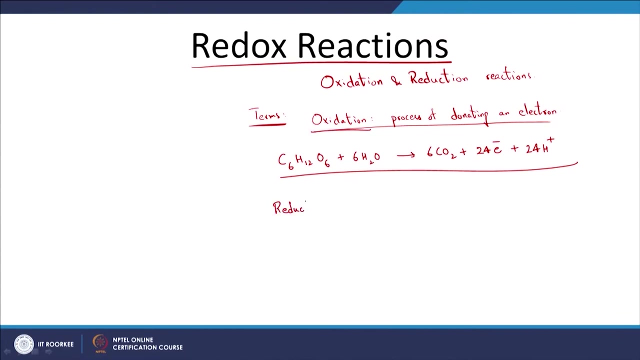 to the glucose or the other. oxidation reactions can be really partial or complete now. So keep that in mind, that the electron release can be either partial or complete here. So this is about oxidation. so if we talk about reduction and it is going to be the inverse, 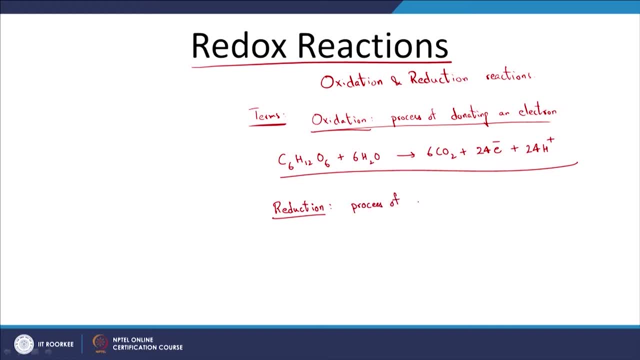 of this process of accepting the electron And relevant example. let us say: you know, let us look at what we usually come across. you know We always have oxygen present in the atmosphere. So let us look at one particular relevant example here. So here we are done with it. so, more or less oxidation process of donating an electron. 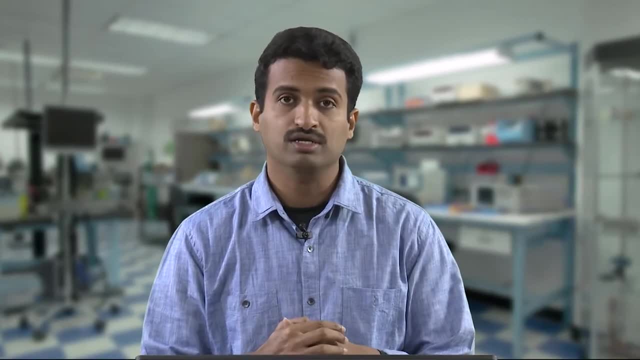 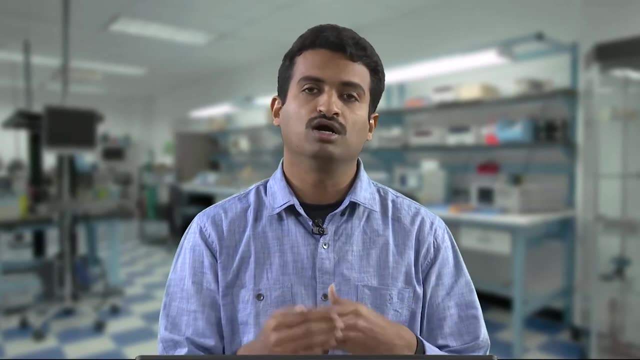 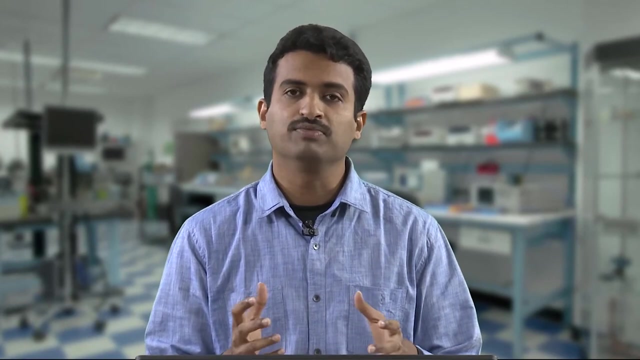 and with respect to reduction process of accepting an electron. So obviously, redox reactions. when we refer to redox reactions, we have both the oxidation and reduction reactions Going through Simultaneously right or occurring simultaneously. yes, So the reason why we stress upon simultaneously is that these relevant half reactions, as in: 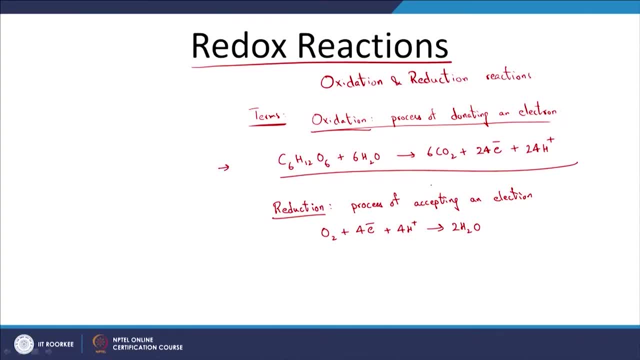 half reactions are those when we write them as the oxidation or reduction. here these are the half reactions where you see either the donation of the electron or the gain of the electron, right, So these half reactions, right, they do not exist in nature, let us say, or in general, out there. 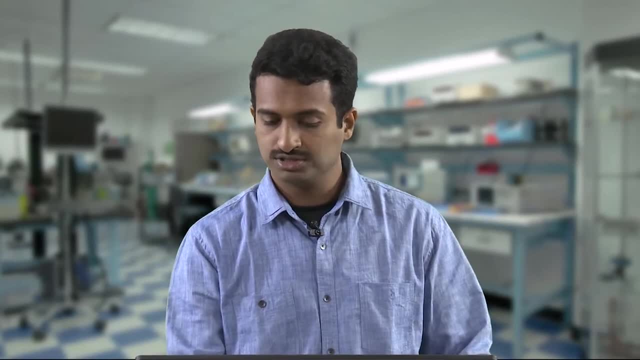 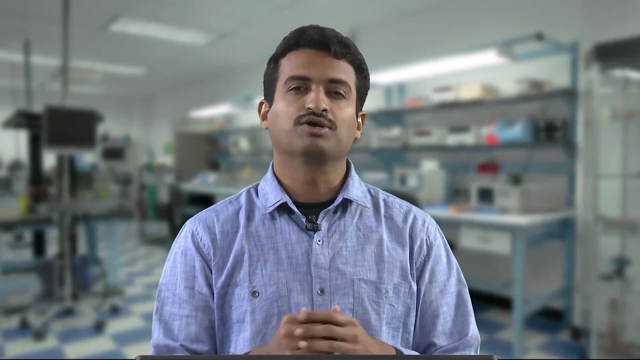 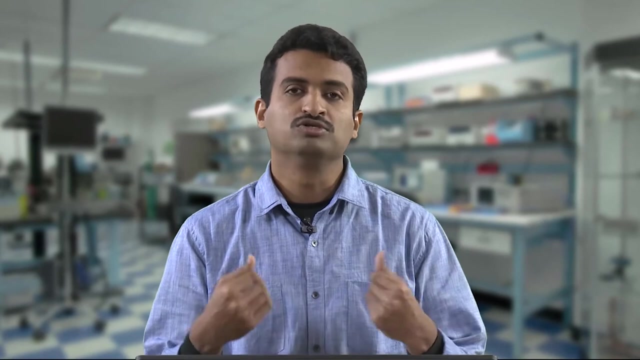 right. And why is that? Because the electrons, They do not accumulate in your particular solutions or such right. So for a redox reaction to go through, the key is that you should have both oxidation and reduction reactions occurring simultaneously, right? So you have a collision, or let us say conductor, right? 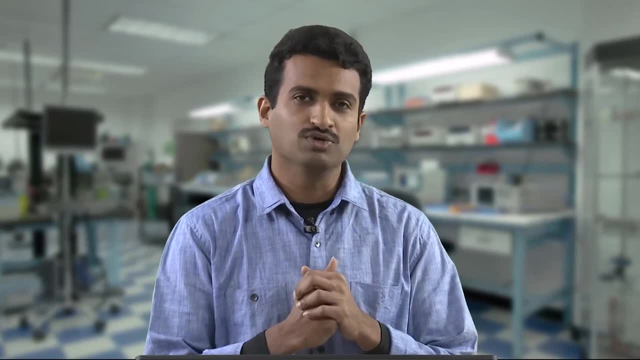 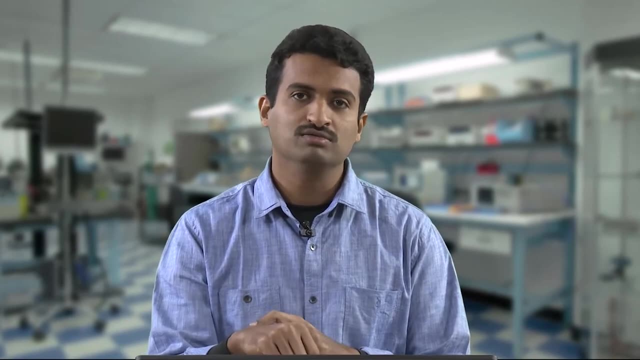 So that you have the transfer of electrons. yes, otherwise you cannot say that. okay, let us say my oxidation half reaction is going to go through, and from time 0 to T1 and from T1 to T2. Then the reduction is going to take place, let us say, based upon the electrons that have. 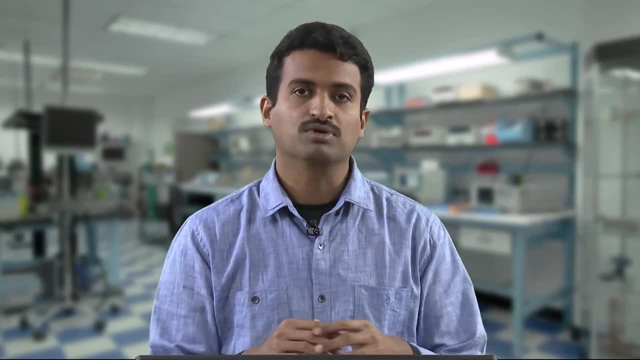 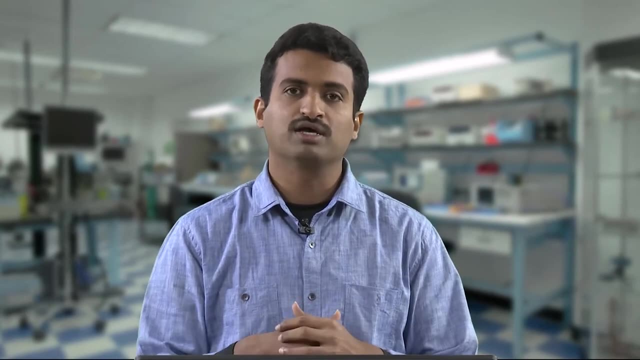 accumulated during 0 to time T1. that does not happen because, you know, electrons do not accumulate in the aqueous solutions, right? I mean, they have half lives, but they are remarkably less So again, for a redox reaction to go through, you will always have both oxidation and reduction. 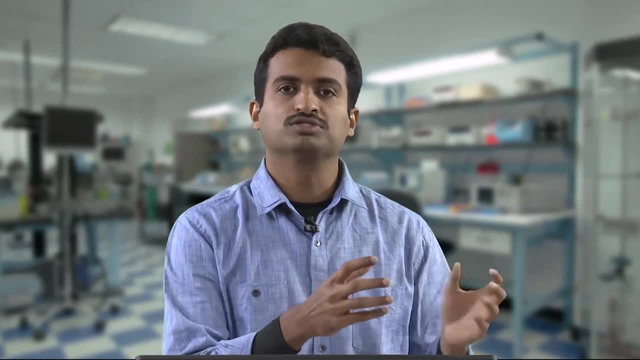 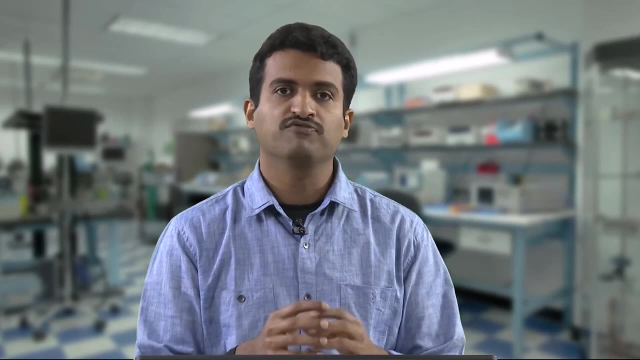 reactions. So. but you usually come across terms like: okay, this reaction is an oxidation reaction, or this particular reaction is a reduction reaction. So what do people refer to? So in that case, people are referring to what is happening, to a relevant target compound in your particular reaction, right? 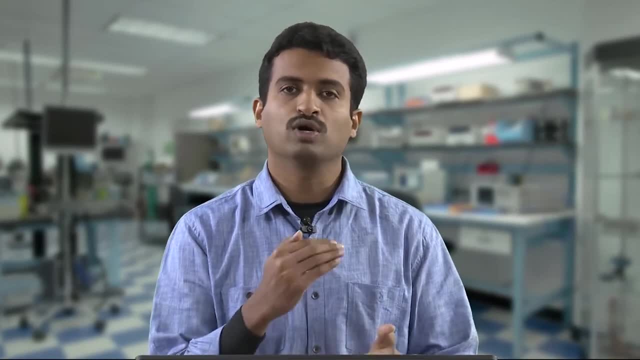 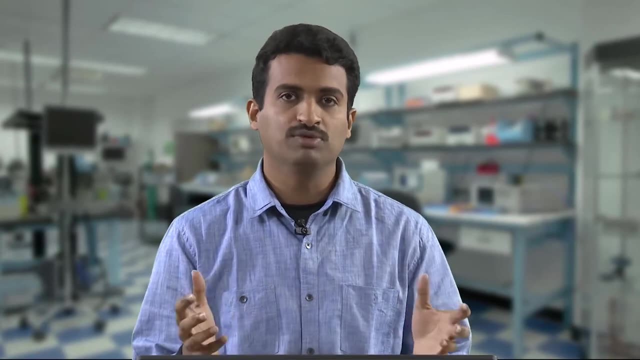 So what do we have now? what do we know? that a redox reaction is one when oxidation reduction obviously happens. I mean, there is an electron transfer right from one compound to the other. and we know that they do not occur independently, they occur simultaneously or in conjunction with. 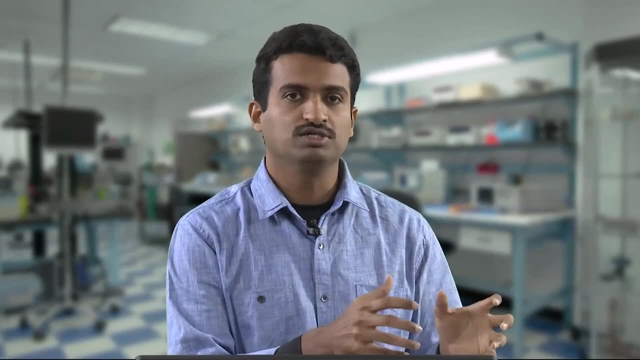 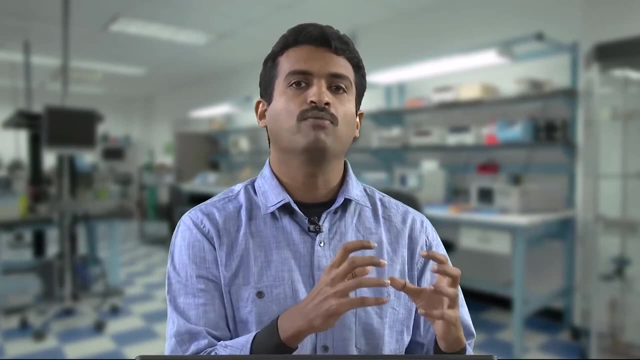 each other right So, but still, people refer to reactions as oxidation or reduction. let us see. but why is that? because, let us say, you are, people are talking about What is happening. What is happening? what is happening to the relevant compound here, Their target compound? is it being oxidized or reduced? and based on that, they look at. 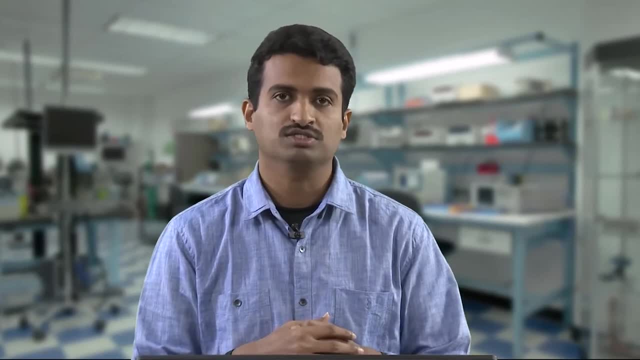 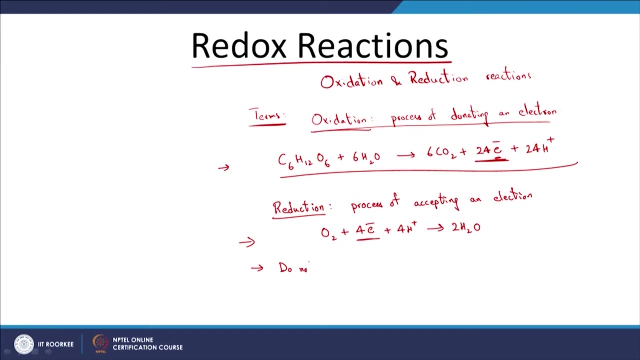 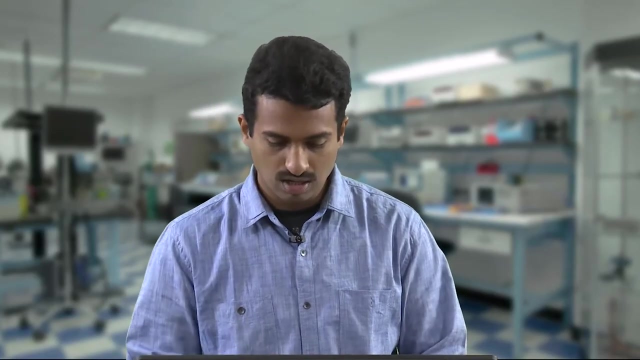 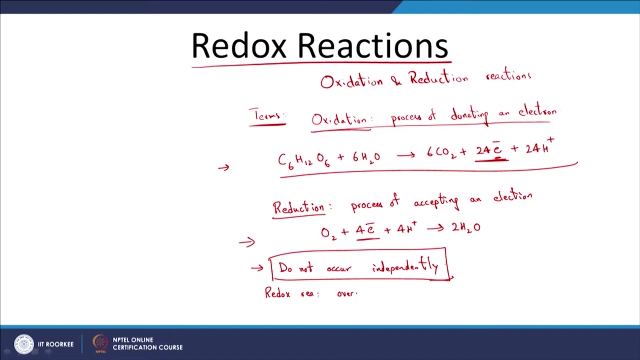 the relevant reactions as oxidation or reductions or such, But keep in mind that they do not occur independently. The whole key is that they do not occur independently. Redox reaction is the composite reaction here. Redox reaction, what is that about? overall transfer, overall process of transfer of electrons? 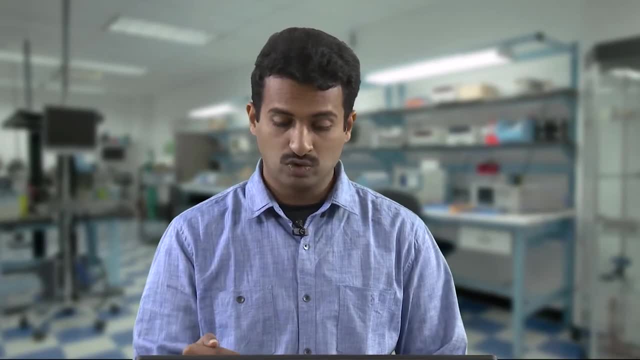 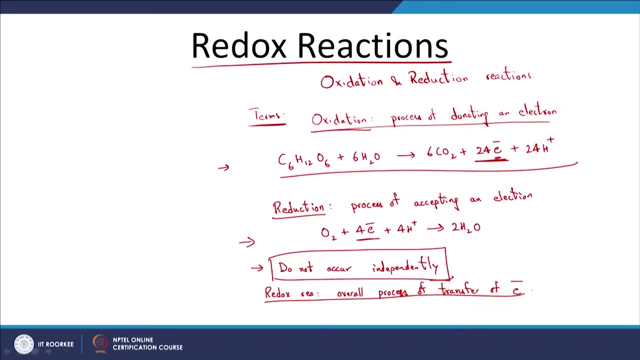 that refers to the redox reaction. We have two particular oxidation and one each of oxidation reduction. Let us look at the relevant redox reaction by balancing the number of electrons, or look at the balance reaction here: C6H12O6 plus 6O2.. 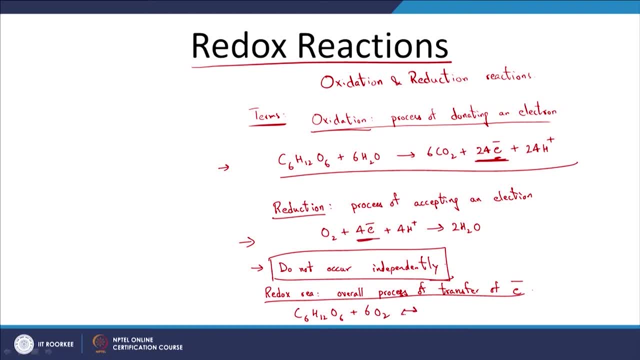 You want to balance the number of electrons will be an equilibrium with 6CO2 plus 6H2O. This is a redox reaction. Redox reaction. This is a reduction half reaction. This is an oxidation half reaction. As you see in the redox reaction, you are not going. 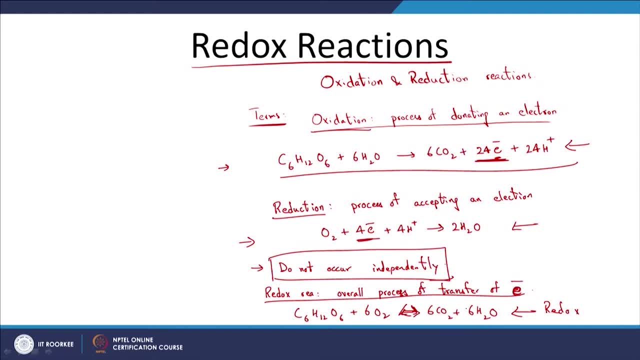 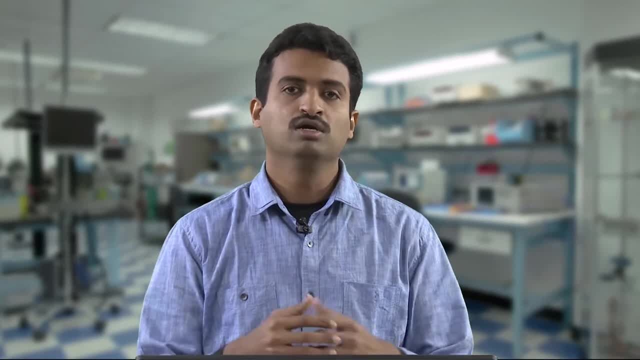 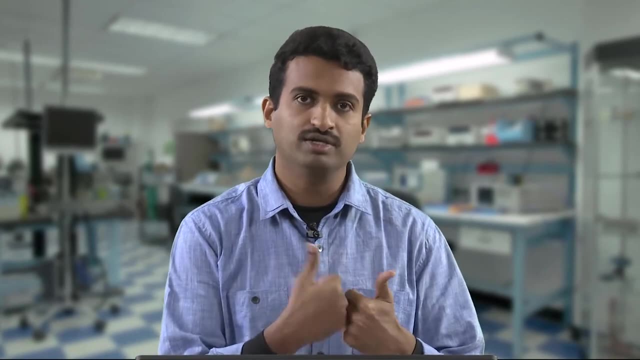 to have, or what is any electrons in the relevant equation? The whole key is that electrons do not accumulate in the solution. Now, how would your redox reactions go through? now? They would go through when one molecule collides with the other, and then there is going to. 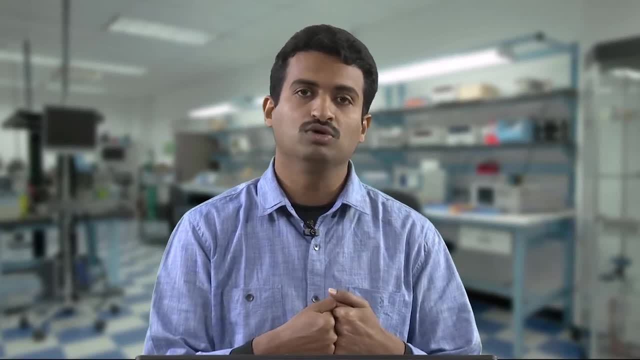 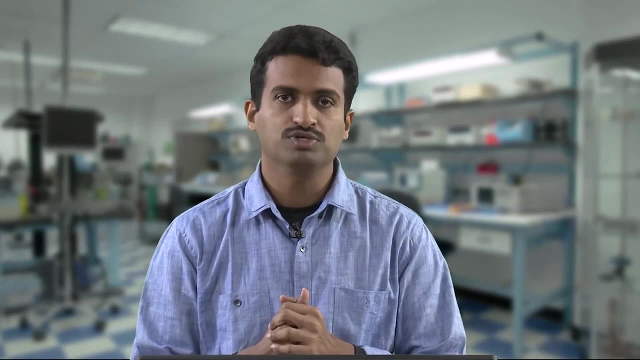 be a transfer of electrons, But when this physical collision of the relevant molecules is not feasible. one other way that these redox reactions can go through is when you have a conductor of electrons. that is what you would see in your electrochemical cells or such. 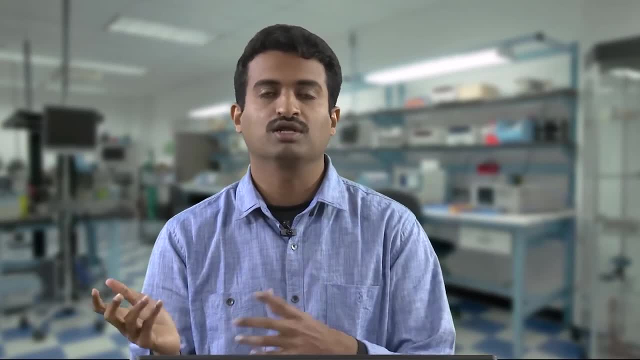 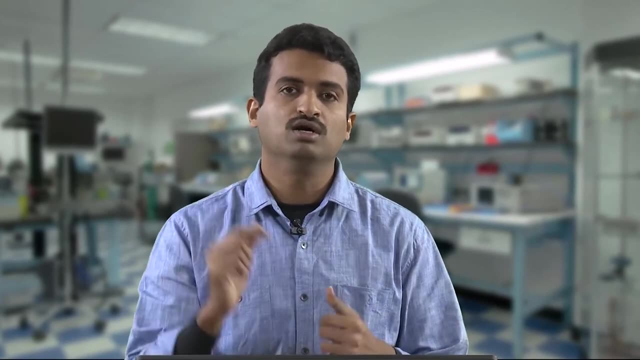 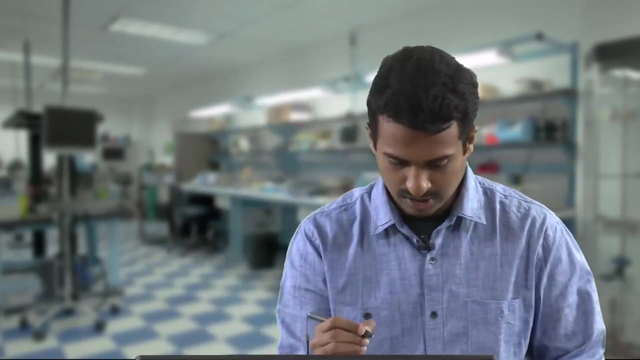 You have a cathode or anode where you have oxidation or reduction at the relevant electrodes, and then you have a conductor. which is what is the purpose of this conductor? for the transfer of the relevant electrons. Let us keep this moving. Let us look at some of the other aspects. 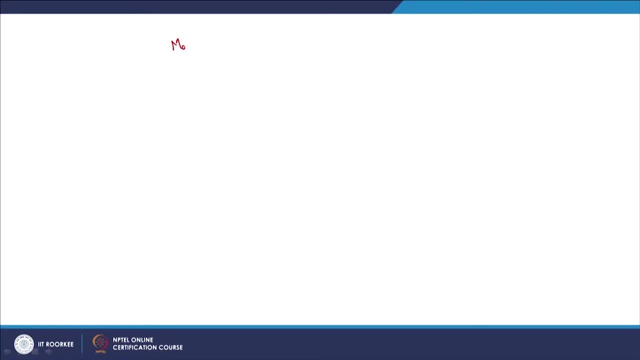 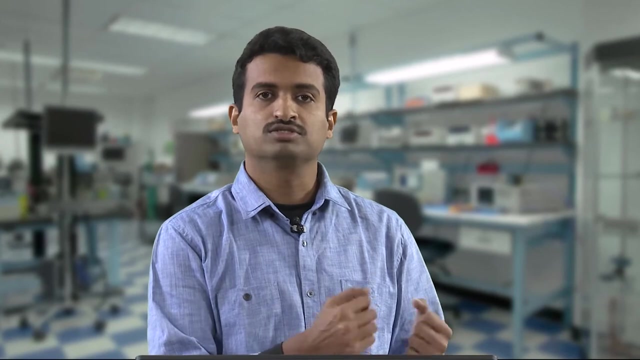 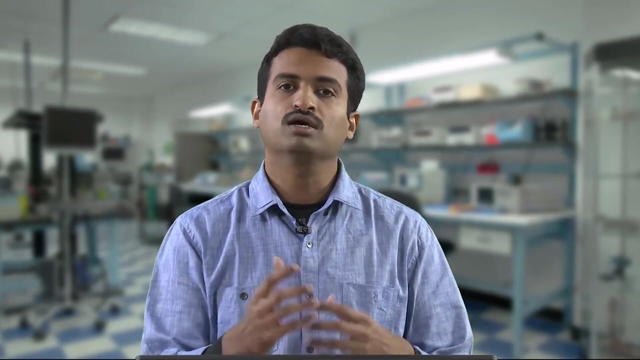 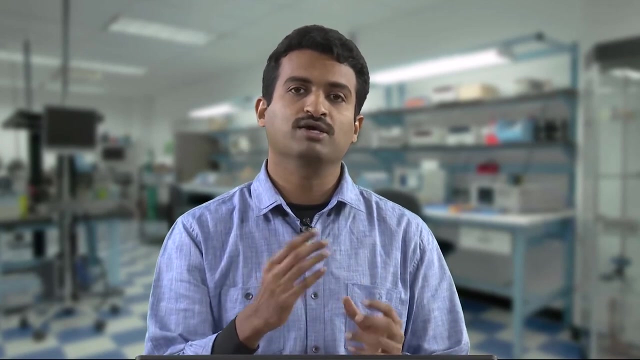 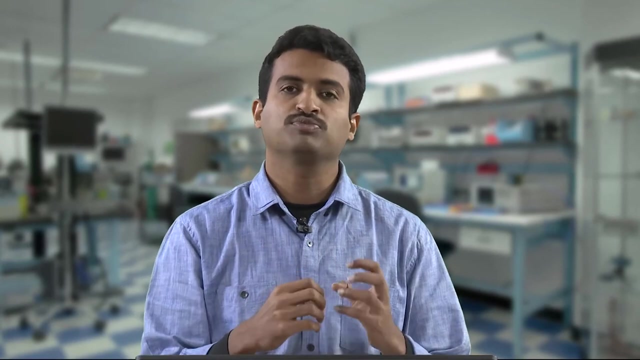 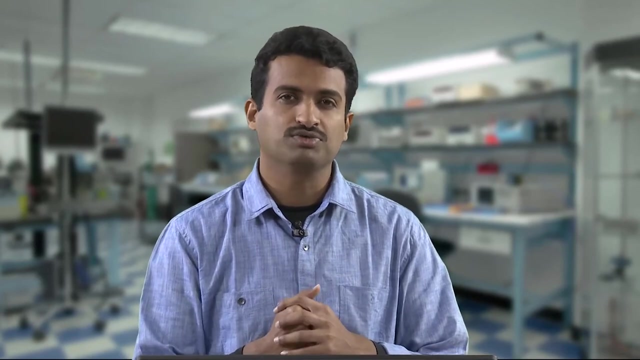 Here we just mentioned that molecule collision is required. and why is that? again, because the oxidation or reduction reactions do not occur. You are going to have a change in the pH. so as H plus increases, pH decreases. and as H plus is removed from the solution or OH minus increase in concentration, you are going 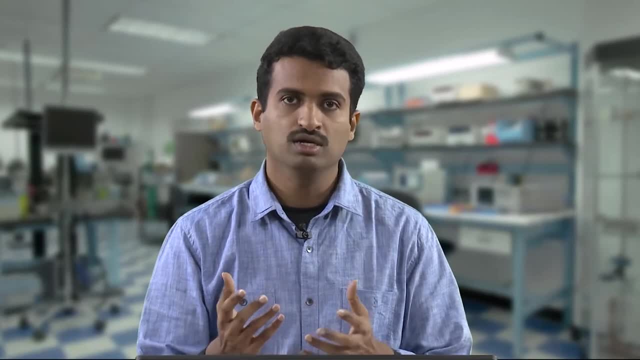 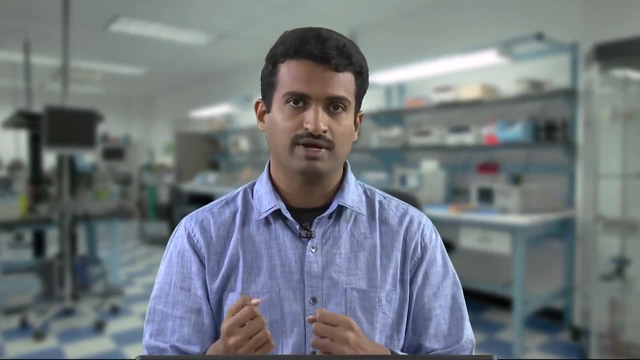 to see a pH. what is increase in pH there, in the acid base? It is an analogous, kind of analogous set of reactions, but keep in mind that, unlike the acid base reactions, you cannot have accumulation of electrons, and that is the key here. Let us move on to some of the other terms. 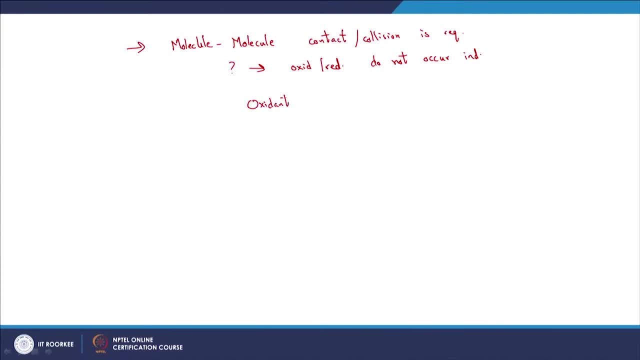 You might have heard, oxidant and reducing agent or reductant, and, in this context, similar to what we have for conjugate acid base pair. for our conjugate acid base, we are going to have a couple here and then we are going to have electron equivalents. 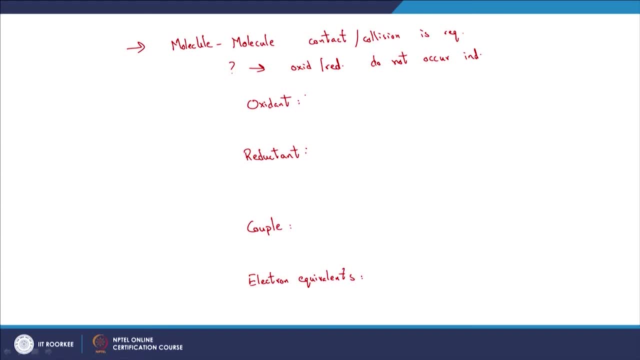 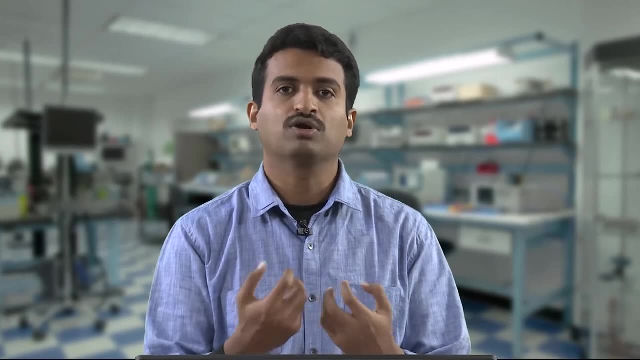 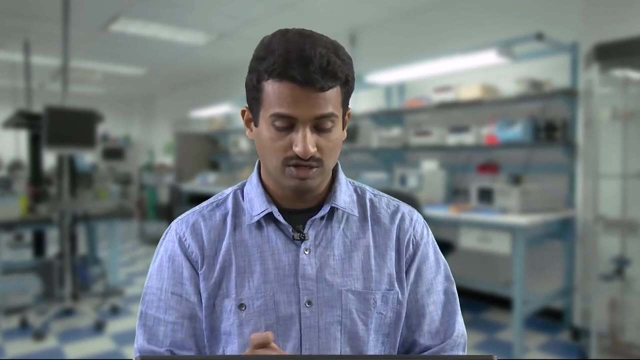 Let us look at what these aspects are For your redox reactions to go through. you have transfer of electrons, so you need compounds that act as electron acceptors and, at the same time, if you have an electron acceptor, you need a compound that would act as a electron donor. 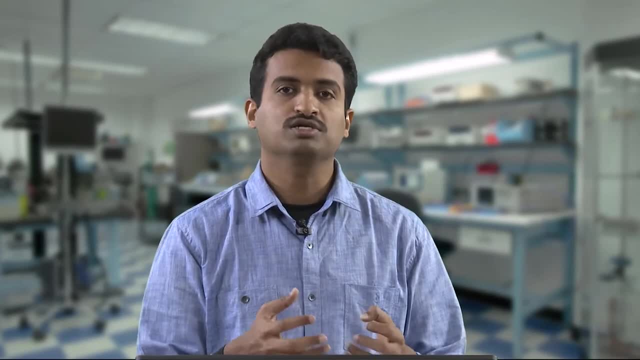 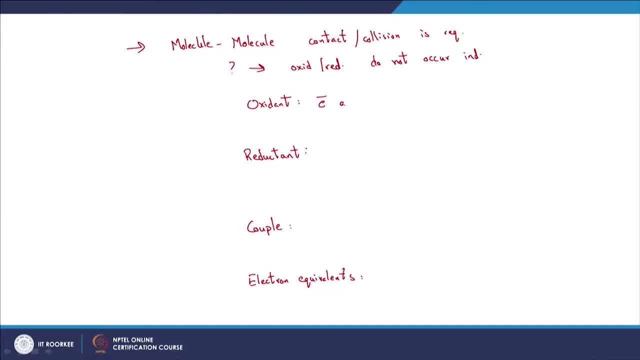 Here we have the relevant aspects or compounds. An oxidant is typically one that would accept electron. so that is now going to be an electron acceptor And, as we discussed, if you have an electron acceptor, there should be a compound available for accepting the, for donating the electron. pardon me, so here, if oxidant is the electron, 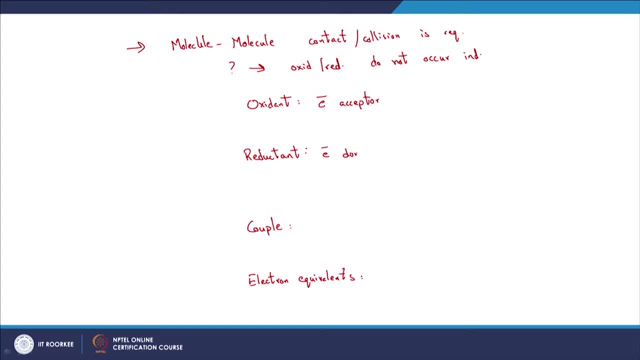 acceptor, reducing agent or reductant, is the electron donor, So oxidant. what does that cause another compound to be? so? it is going to oxidize the other compound. So again oxidant. an electron acceptor: it is accepting the electron. so in that process, 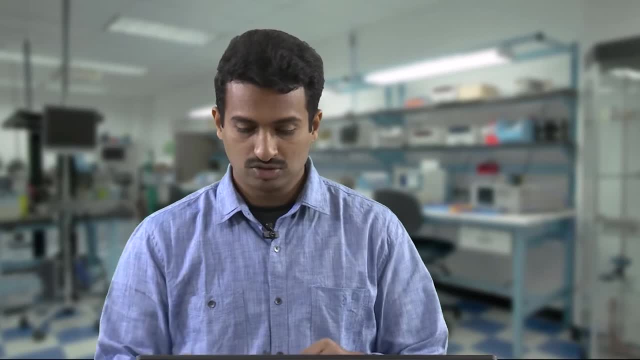 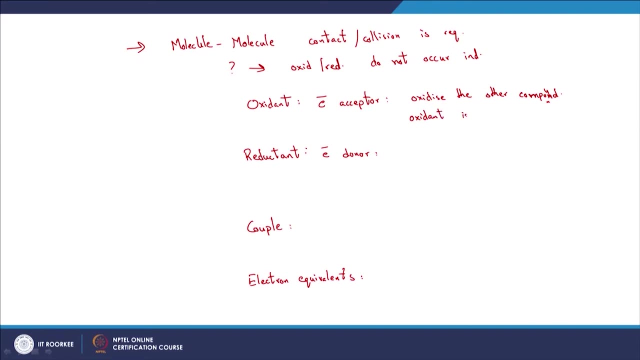 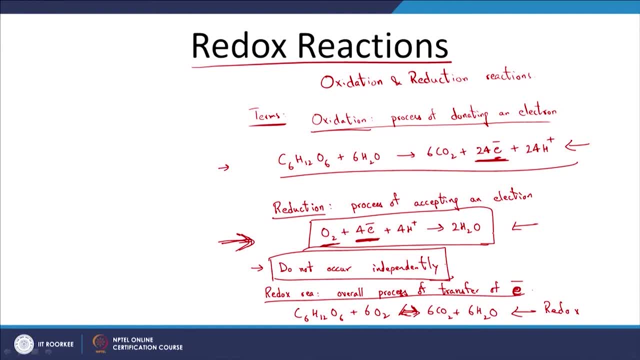 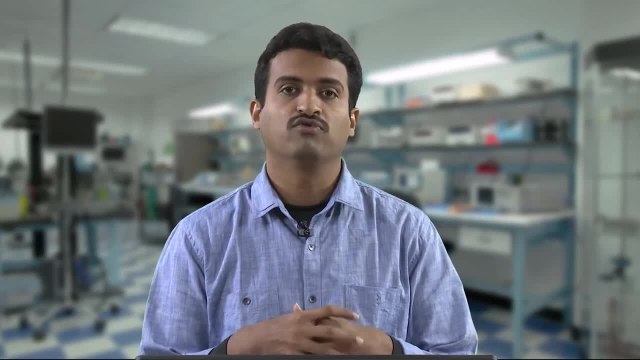 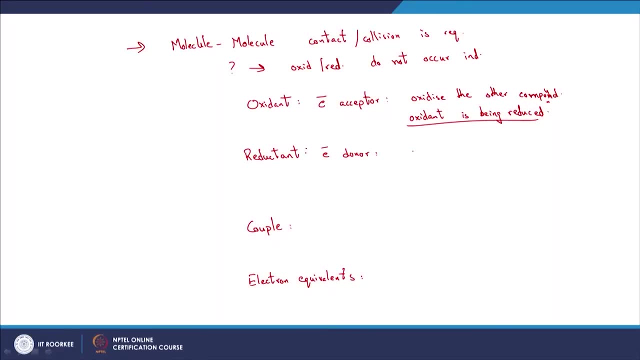 Here is a relevant reaction we see out here and in the process of accepting relevant electrons, or the electrons, which are four electrons, we see that it is being reduced. so we are done with that. and reducting, obviously it is going to reduce the other compound, other compound, 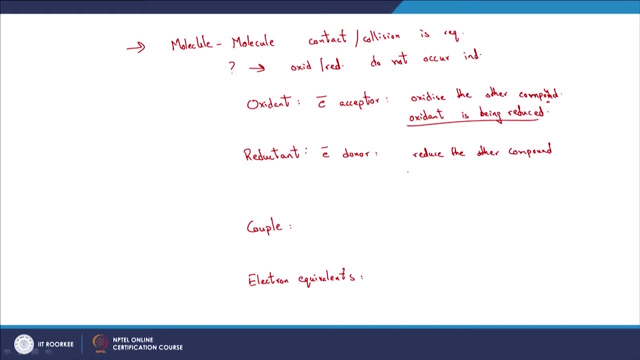 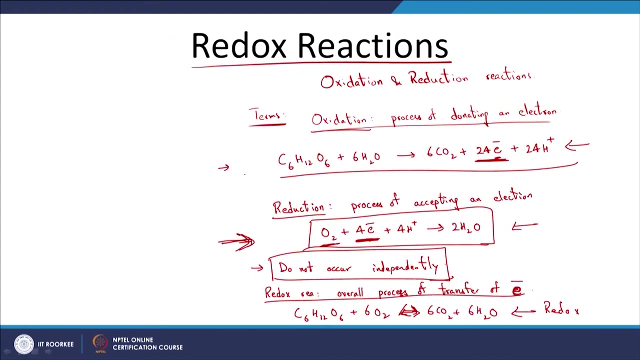 And let us look at the relevant reaction again that we had earlier. and the reducing agent, or reductant, is in the process being oxidized, right, and let us look at what we have just described here. So here this is the relevant reaction. let us say- and now obviously you see that this: 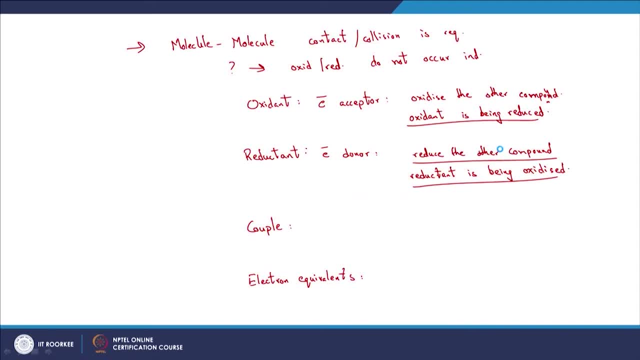 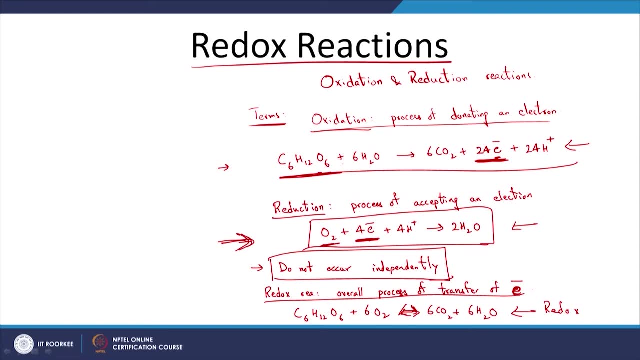 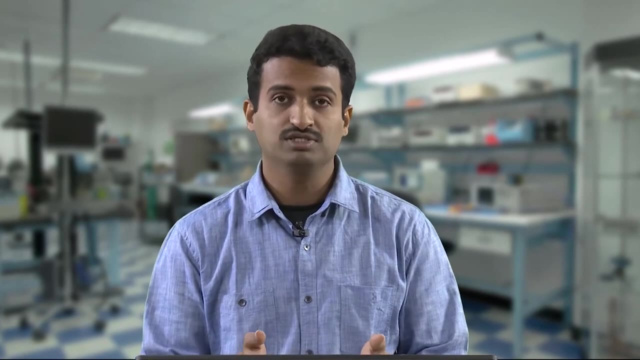 glucose can act as an electron donor, and which is what we just described here. So thus, in this particular case, glucose or C6H12O6 is a reducing agent or a reductant right. So reducing agent is one that would donate the electrons right, and in this case we see: 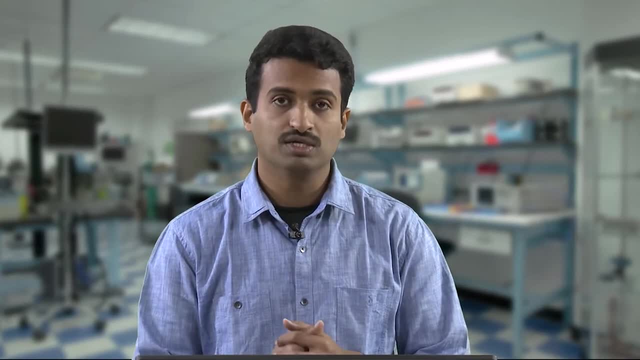 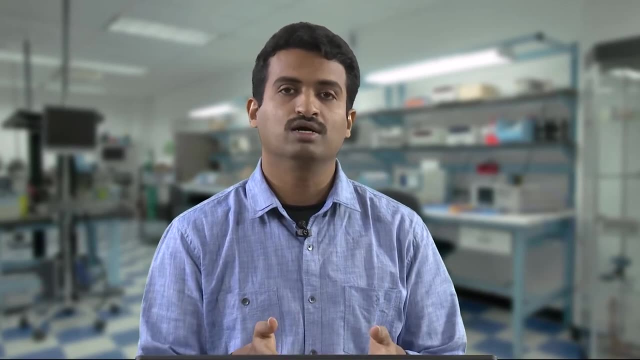 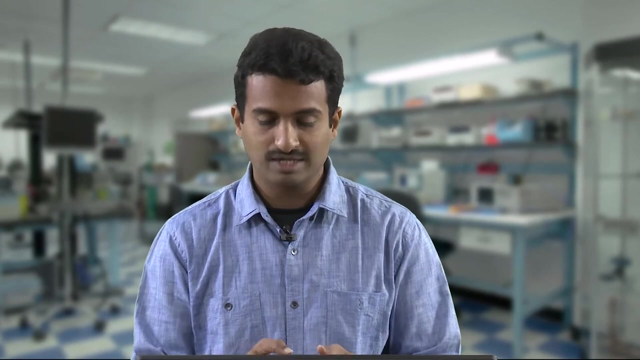 that the relevant, what do you say? half reaction. if you look at the relevant half reaction, we can see that glucose can- what do we say? donate the relevant electrons, right? So that is why, in this particular context here, I guess glucose is a reducing agent, right, but as you see in this process, right, it is. 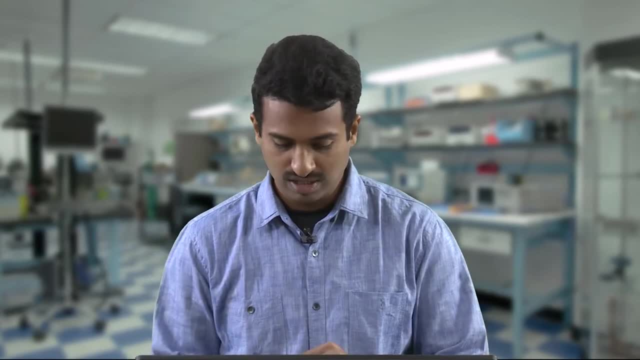 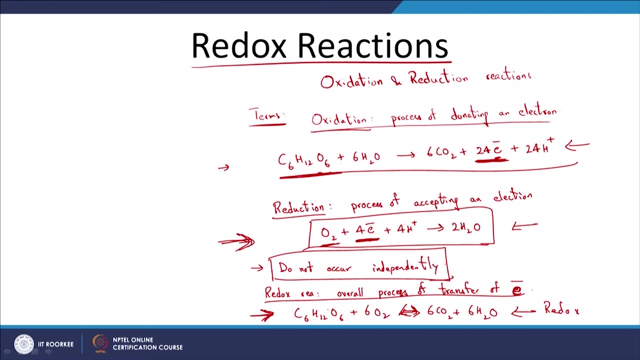 being oxidized. glucose is being oxidized, right? So that is what we see and obviously, if you look at this particular composite reaction or the overall reaction, I guess what do we see here with respect to this particular case? oxygen is oxidizing your particular glucose molecule. so oxygen, which is an oxidizing agent, 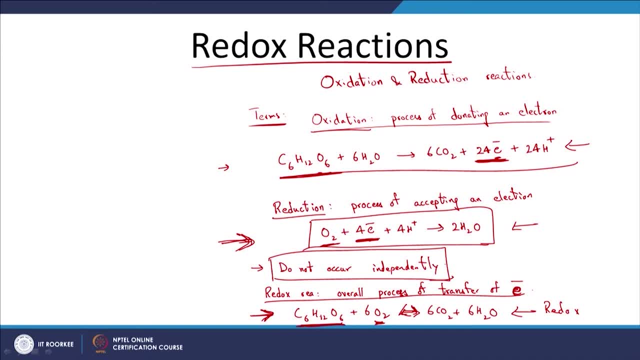 is oxidizing your particular compound compound, which is glucose in this particular case, while being reduced. so that is what you see here. So oxygen is acting as the electron acceptor, glucose the electron donor and in general, because, let us say, we are our target compound here, is this particular glucose molecule. 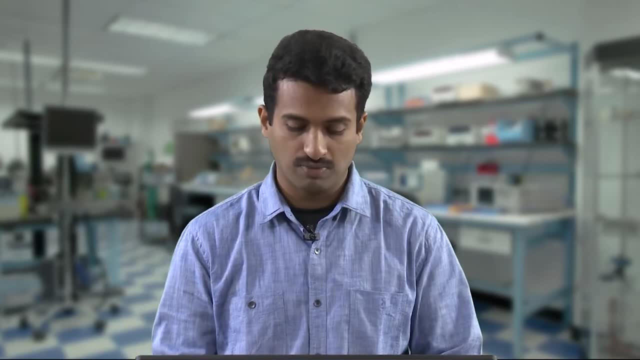 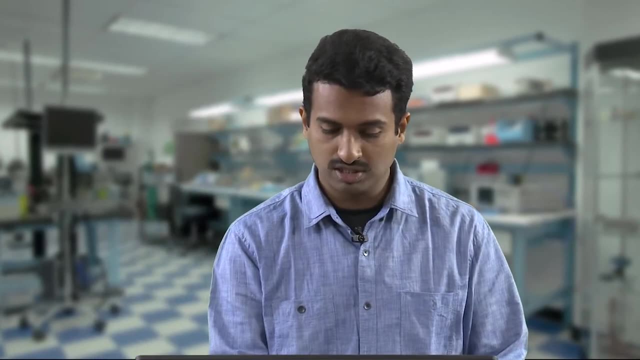 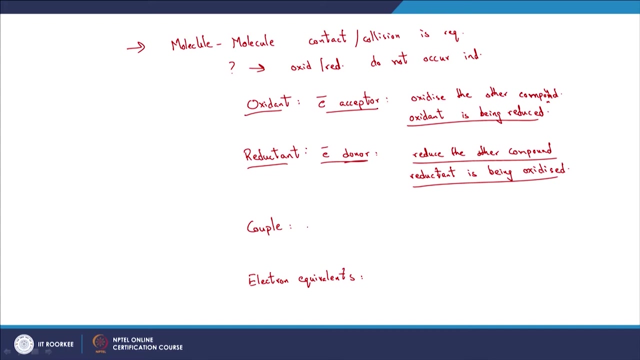 So we refer to this particular reaction as oxidation, but in general, as you see, you have both oxidation and reduction occurring simultaneously. So that is one particular aspect. here again, oxidant is an electron acceptor, reductant is an electron donor. So couple, I guess, so similar to the conjugate acid base that we have looked at earlier. 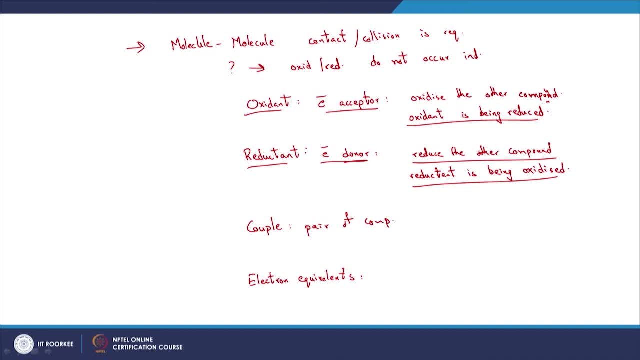 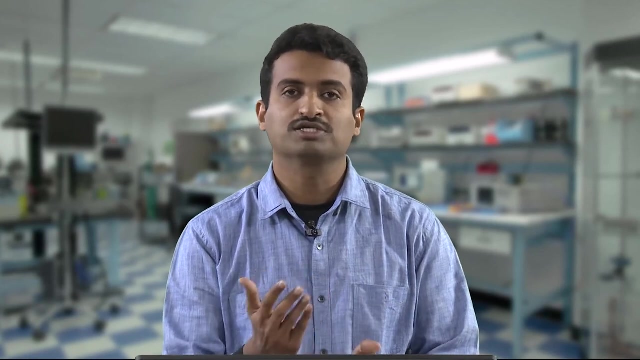 So we have this pair of compounds which would represent before and after exchange of electrons, so similar to the conjugate acid base pair, which are the compounds before and after exchange of the proton, Or H. plus here we have what we say a couple redox couple, a pair of compounds which would 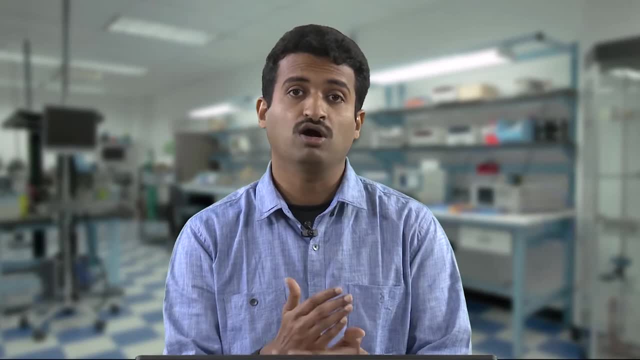 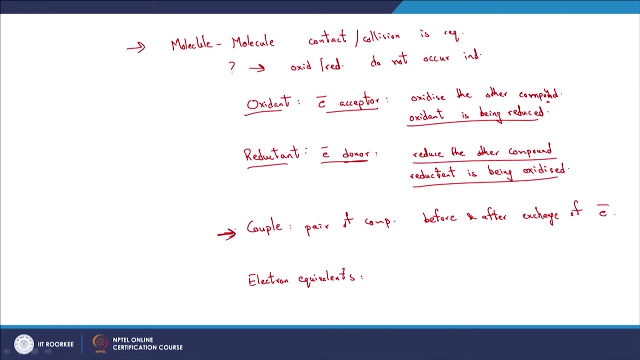 represent. what do we say before and after stages of electron transfer? So obviously here I guess there are different types of couple, different kinds of couple, so we will come back to that later on. So again, one aspect here is that we need to keep in mind is equivalents. so we talk about 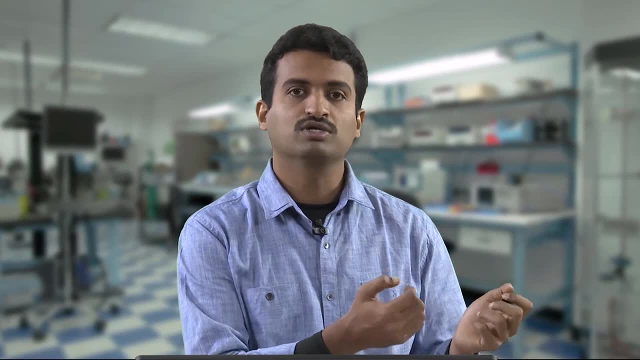 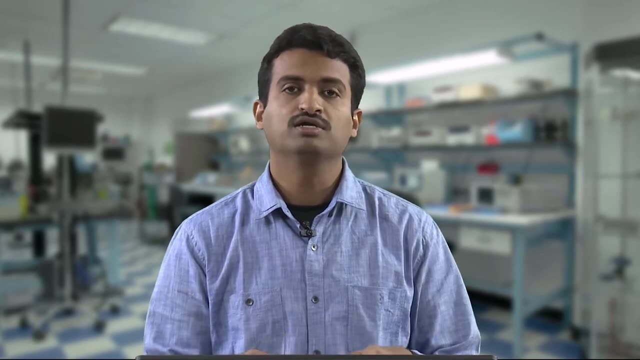 equivalents, or we talked about or looked at different aspects with respect to equivalents earlier, but most of them were with respect to charge. let us say, Most of them Coming, And here also we have a relevant concept of equivalent. but here we talk about electron equivalent, not with respect to charge. 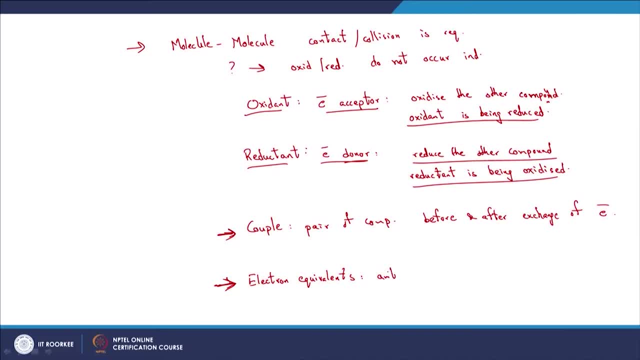 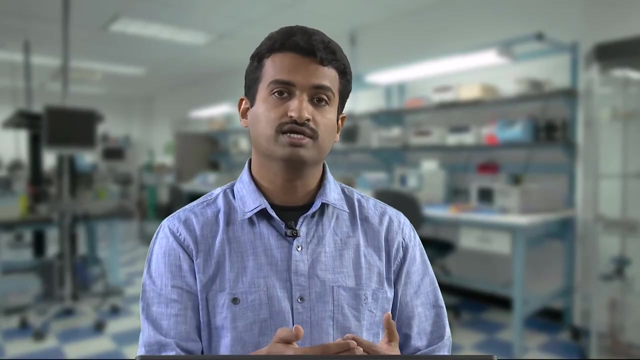 But I guess the concept is similar. It is the amount of material that will donate or accept one mole of electron. now let us talk about electron equivalence: Honey, Yes, Okay, Okay, Okay. electrons With respect to charge: we define it in terms of per mole of the charge and 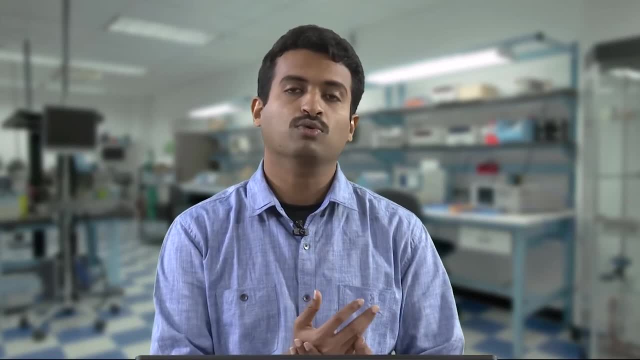 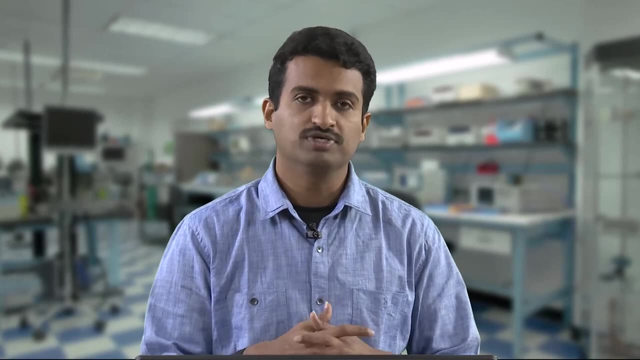 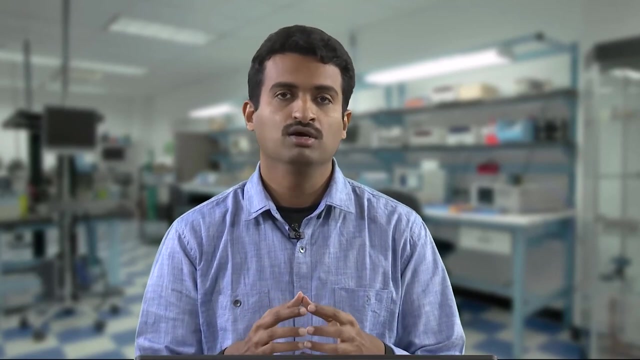 here we are looking at compound that will either donate or accept 1 mole of electrons that we would refer to as electron equivalents. There is a particular example we are going to look at with respect to COD test, as in COD it is the chemical oxygen demand, but you are using potassium dichromate to be able. 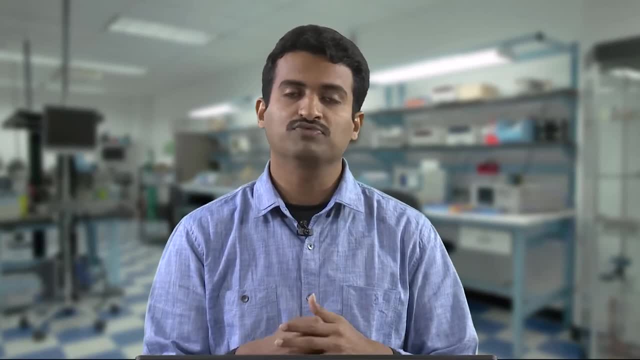 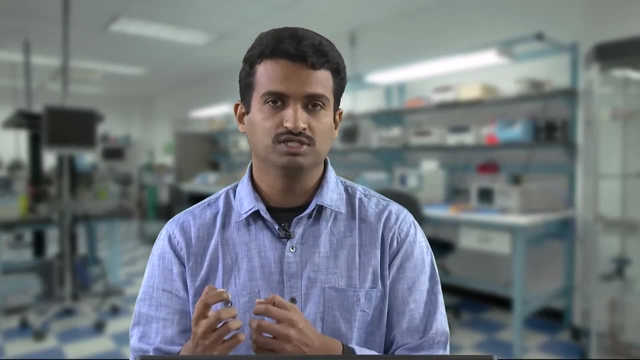 to measure this. There is going to be a transformation in the relevant units from the chromium or dichromate that you measure for its loss to the oxygen demand. That is what we are going to look at later on and in that context we are going to look. 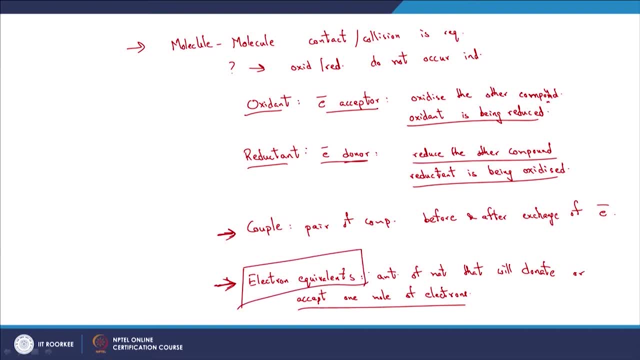 at electron equivalents later on. But one aspect with respect to electron equivalents is that we are talking about electron equivalents now And keep in mind that it can vary. now, why is that? because different compounds, for example. look at this particular examples. with respect to sulphide, we have this particular case and 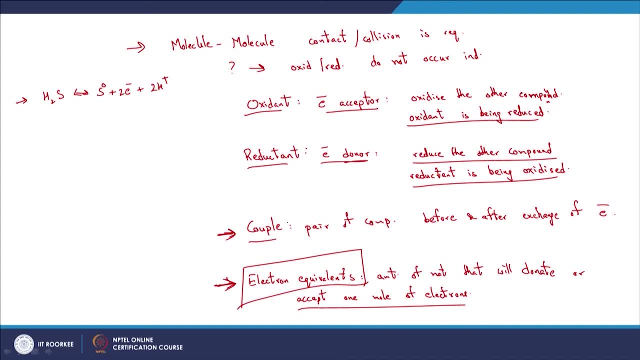 from this particular aspect, you can identify one set of couple, but keep in mind that the hydrogen sulphide can also. So let us discuss this with respect to crockery. and now, 5 moles of electron equivalents is one example of test like this. we were talking about that: toxinated provisionances, which 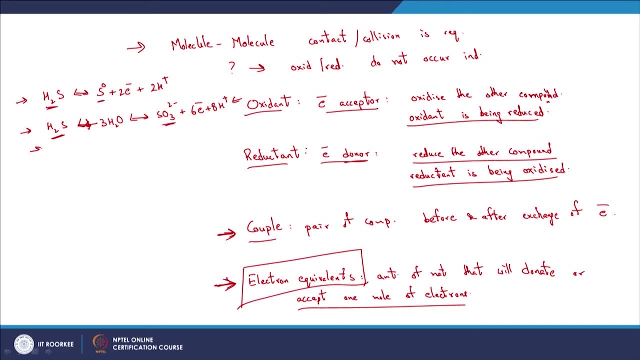 we are just going to discuss later on And after in particleTomato anyway, there is cascade. talked about stationer, here you can see about a abundance, but then They are called hydropt tails, gas plus tan, H plus. so here we are. come across examples, three examples wherein the couple 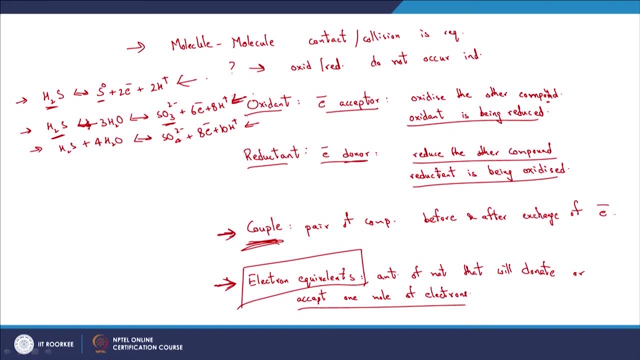 we have the couple and it is depend upon the type of half reaction. So, in this particular case, what is the couple? H2S and sulfur, and the second case, H2S and SO3 2-. and in the third case, the couple is H2S and SO4 2-. so the reason why we looked 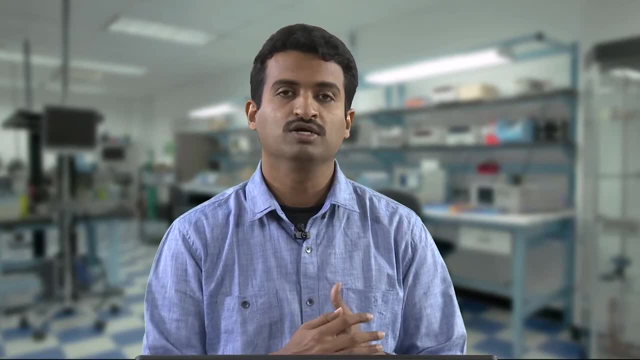 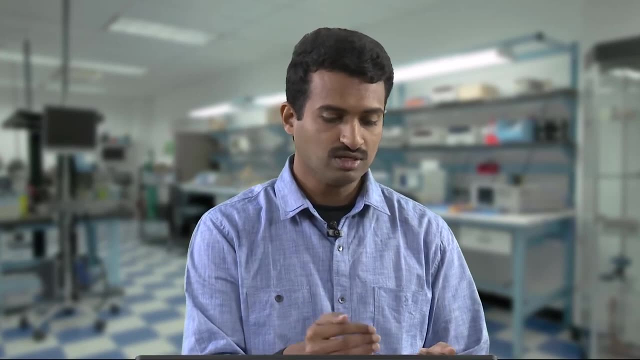 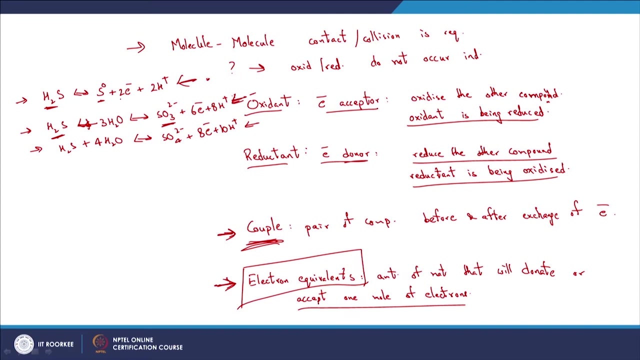 at some of these example is that when we are looking at electron equivalents, it also depends upon the half reaction that you are looking at. So, for example, the number of moles that is being donated for H2S is different for this particular reaction and it is two electrons here and it is different here because it is 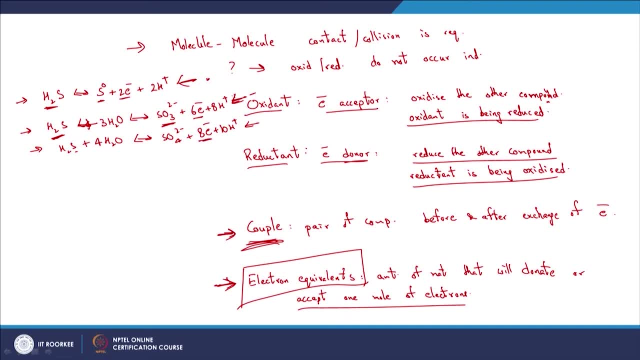 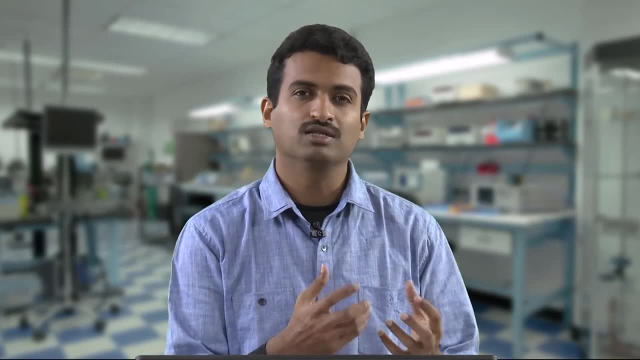 six electrons here and different here in the third case, because it is eight electrons here. So when you are looking at or defining the electron equivalents, as in the two electrons amount of the material that will lead to loss or gain of one mole of your particular, what? 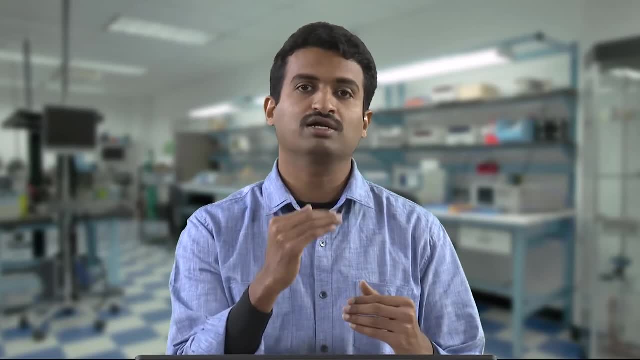 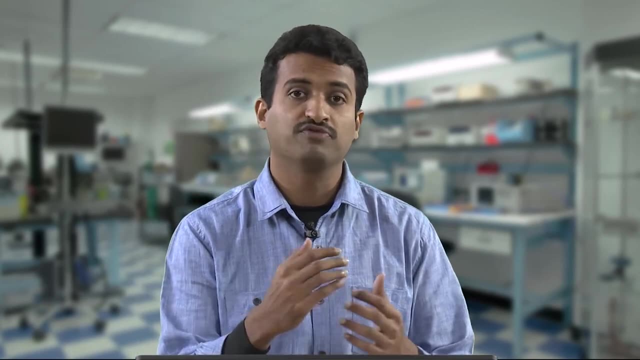 is this now the electrons. So you need to look at or consider that relevant half reaction because for same compound or molecule you can have different kinds of half reactions or different half reactions, leading to different electron equivalents here. so that is the reason that why we looked at this. 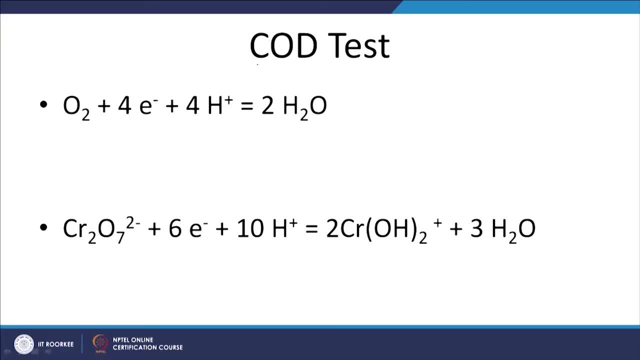 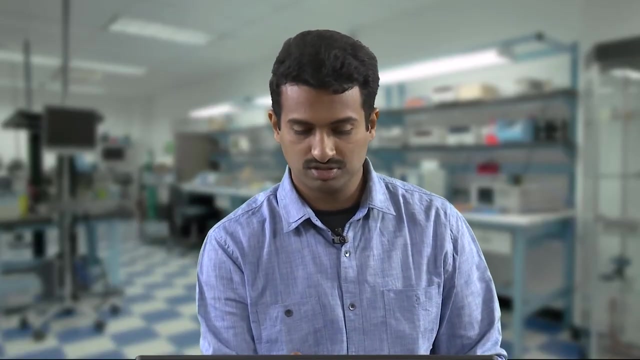 particular set of examples. So we will now move on to applications And, in this context, let us Go ahead and look at this particular COD test that we talked about earlier, and I want to talk about it in the context of the electron equivalents. So what is this particular COD test about? now we know that this is the chemical oxygen. 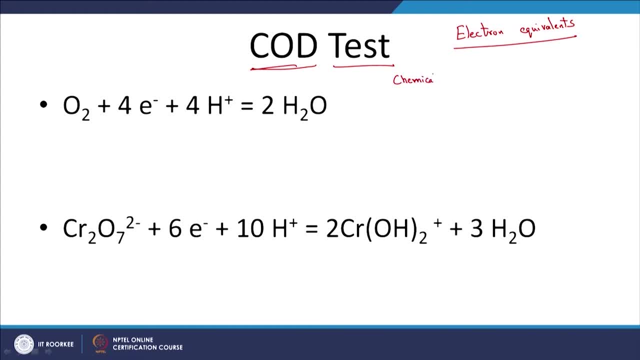 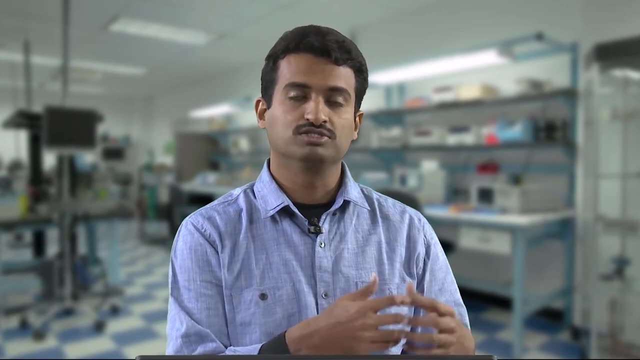 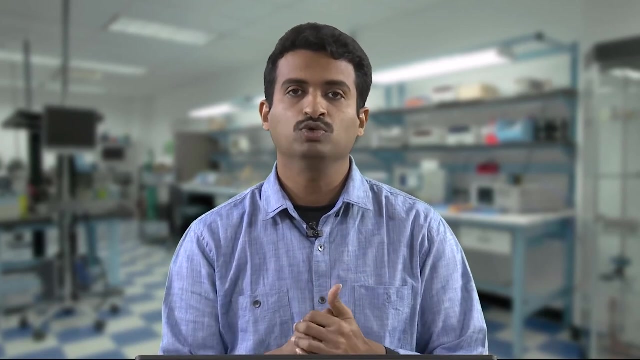 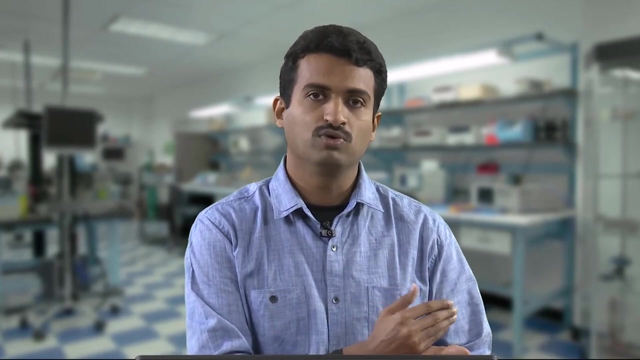 demand. If I have a certain kind of waste, I want to know because if I discharge it into the waters and it can consume the oxygen- dissolved oxygen- in the water, so I want to be able to get an idea about its oxygen demand. So in that case people look at biochemical oxygen demand, the BOD or COD2, chemical oxygen. 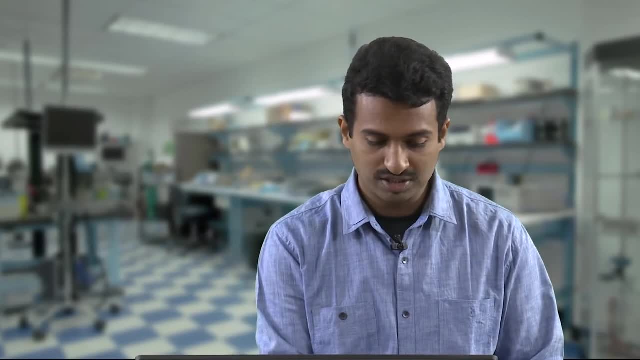 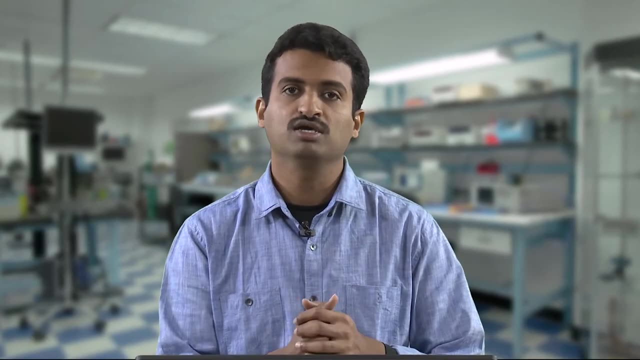 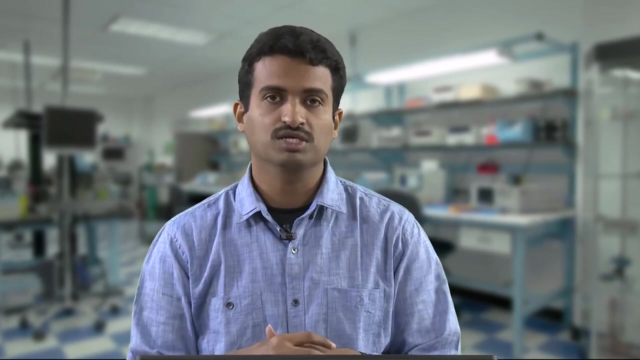 demand. So I guess we are trying to understand the amount of O2 That this particular Material or the waste would consume if it was let out into the streams or into the nature. But COD is chemical oxygen demand. both biodegradable and non-biodegradable fractions are going to 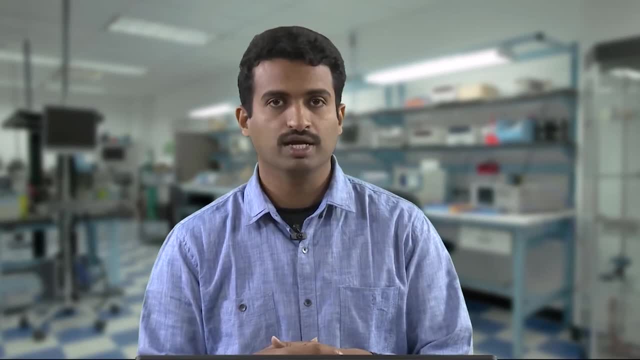 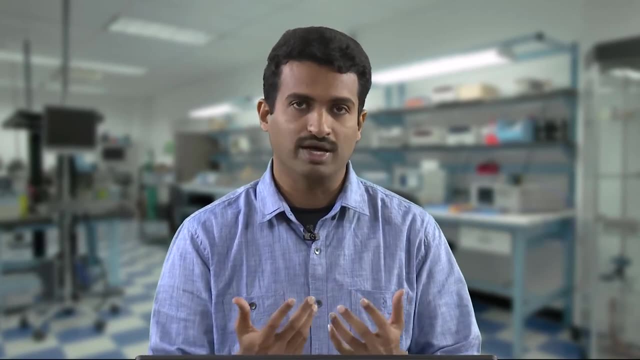 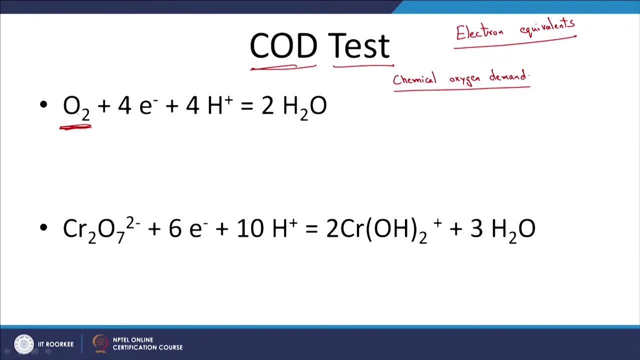 be considered or looked at in this particular experiment anyway. so we are trying to understand: how much oxygen will this particular material require or consume? and what do you mean by consume? for example, here we know that Oxygen is an electron acceptor. so the waste that we are looking at, we are more or less 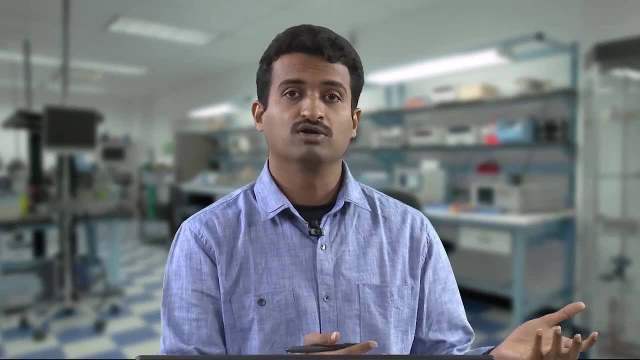 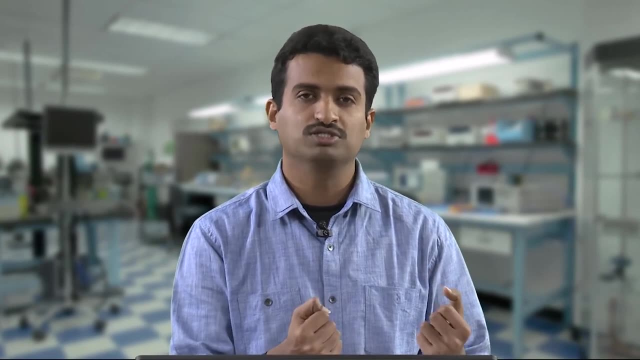 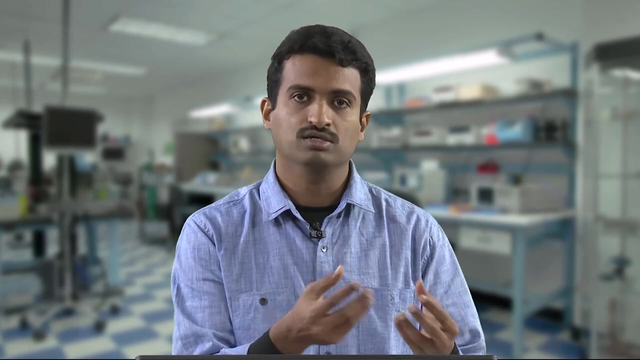 I guess we have reduced forms of carbon in our particular waste water anyway, and there are other examples too. So you have a reduced form of carbon and you have an electron acceptor on an oxidizing agent which is oxygen. So this particular oxygen will oxidize your particular waste, that or sewage that you let. 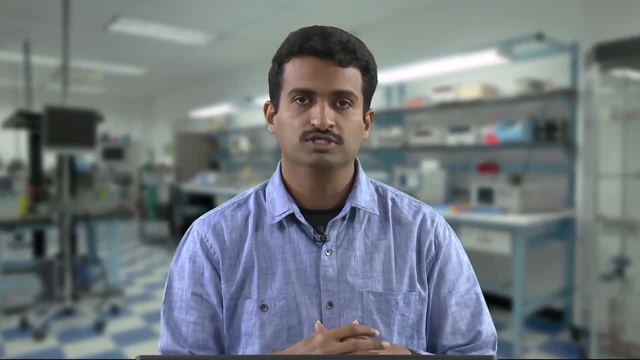 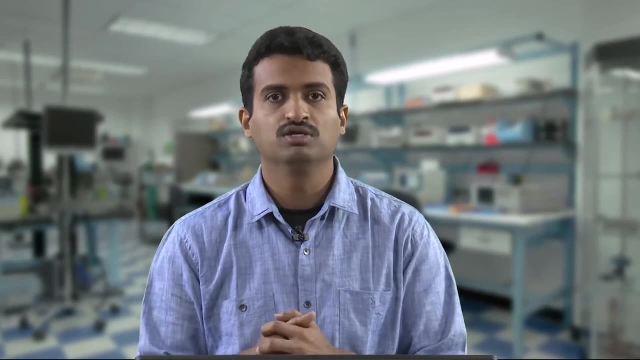 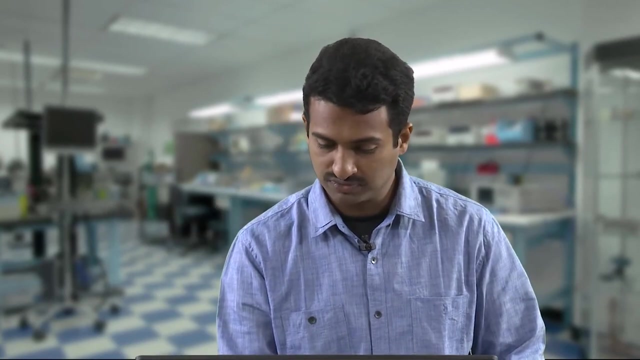 out into your particular nature. Yes, So We are concerned with how much oxygen will this particular waste or stream consume, because, obviously, if the dissolved oxygen falls below certain thresholds, you are going to affect the aquatic ecosystems. So what are we doing this particular test for? to be able to measure the biodegradable 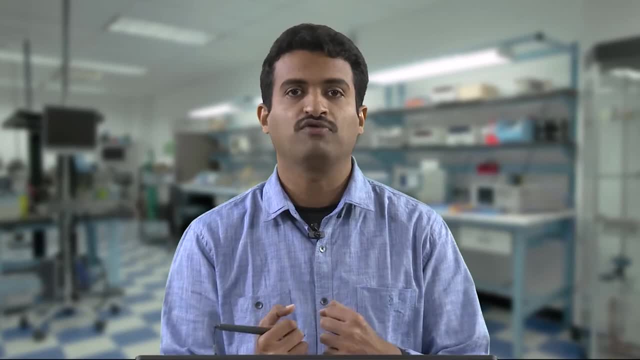 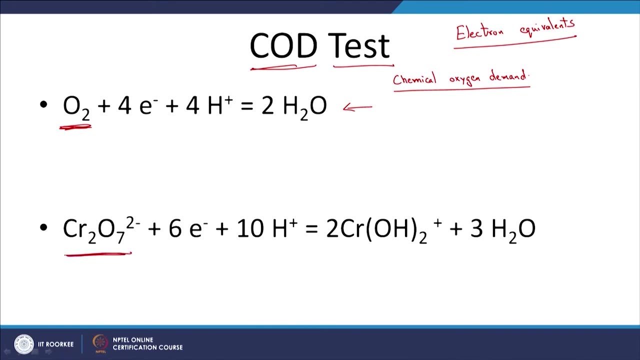 and non-biodegradable fractions in terms of the amount of oxygen that they will consume. but how do we do this test though? So we add potassium, or the dichromate in the form of potassium dichromate in your particular. what is it now? 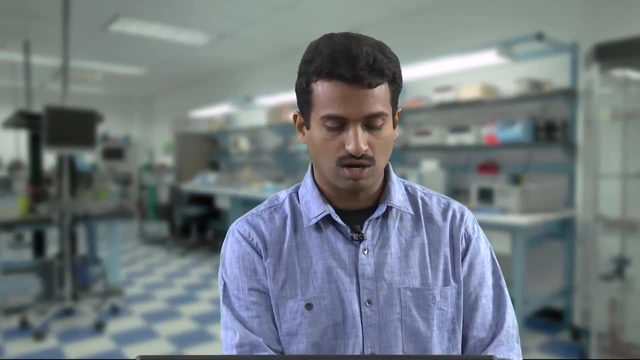 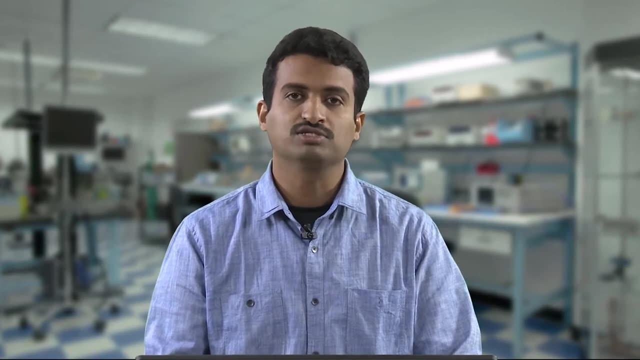 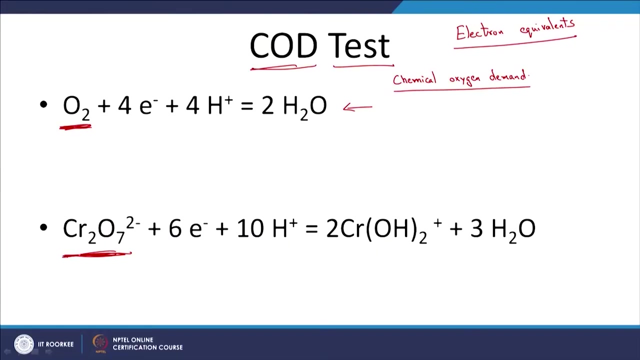 Experiment. so why it is that this is a strong oxidizing agent? if I wanted to conduct the test with O2, the kinetics would be so slow it would take for considerable time or impractical or infeasible amount of time. So we are going to add an oxidizing agent- strong oxidizing agent, pardon me, and that. 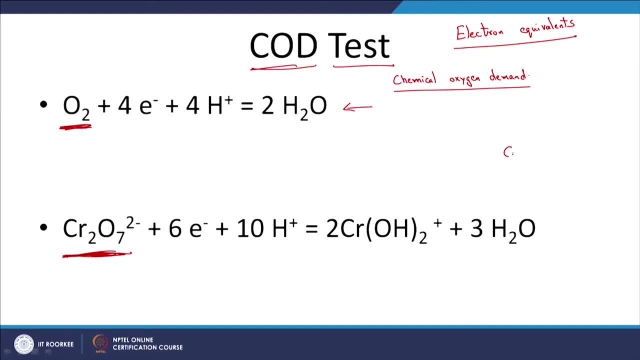 is going to be Cr2O7, 2- and we are also going to add a few catalysts. yes, we are going to add catalysts too. Yes, And obviously, I guess heat it up to. you want to increase the rate of your reactions and 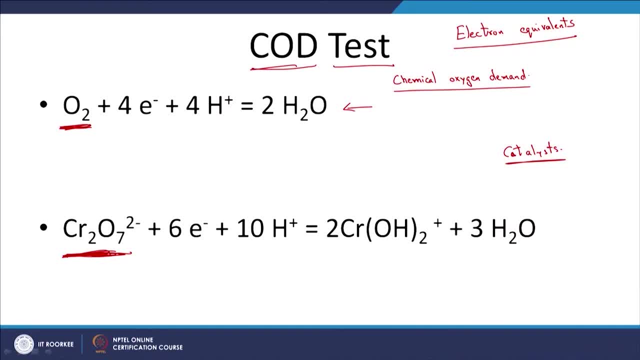 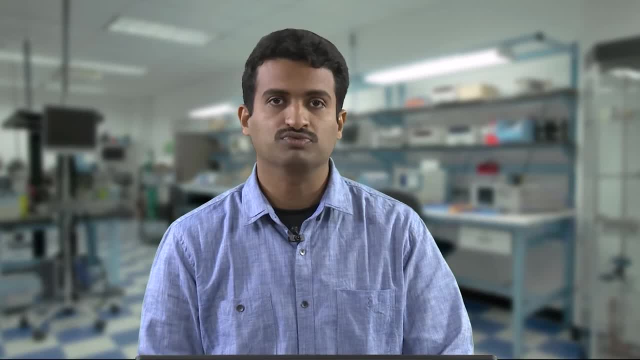 such, and what is the role of this dichromate here? as you see, it is accepting electrons. it is similar to oxygen, it is an oxidizing agent, or it can accept electrons from your particular waste that you are talking about, which is either your biodegradable or non-biodegradable. 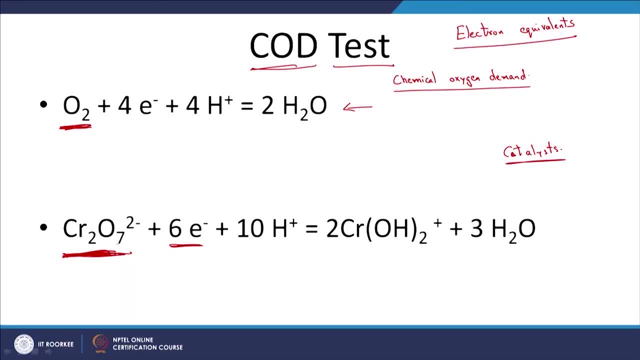 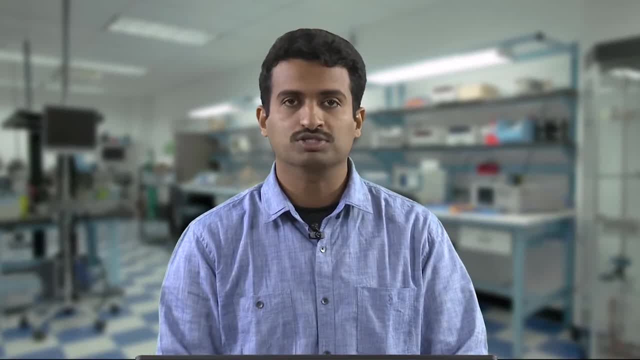 compounds, but here, because this is a strong oxidizing agent and we are going to look at later on why we call a particular compound a relatively strong oxidizing agent or a particular compound a strong reducing agent. I mean, there should be similar to what we discussed with. 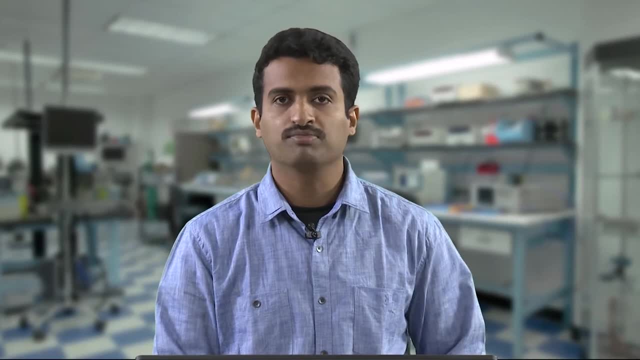 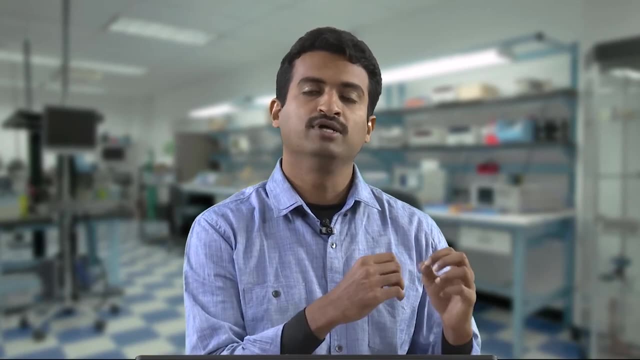 respect to acids, as in we had strong acids or strong bases, or weak acids and weak bases, and so on. So in this case too, we are going to look at, I guess, relevant similar aspects. we are going to have strong oxidizing agents or, you know, strong reducing agents, but again, keep in mind, 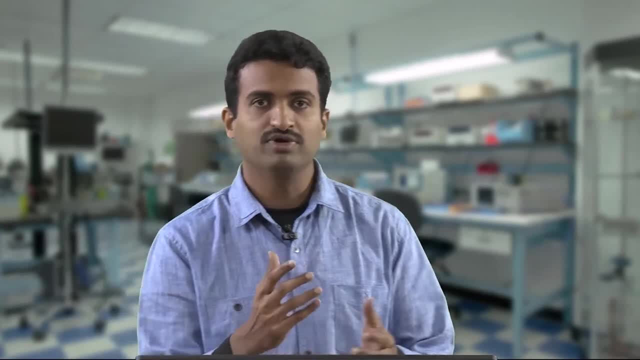 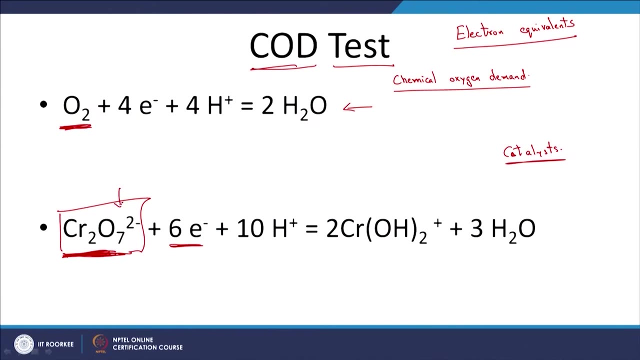 that all these are relative, So we are going to look at the relevant redox potential or such, Yes, Later on. though, again keep in mind that we are just adding a strong oxidizing agent in the form of Cr2O7 2-, so it can take in a certain number of electrons, and this is your relevant. 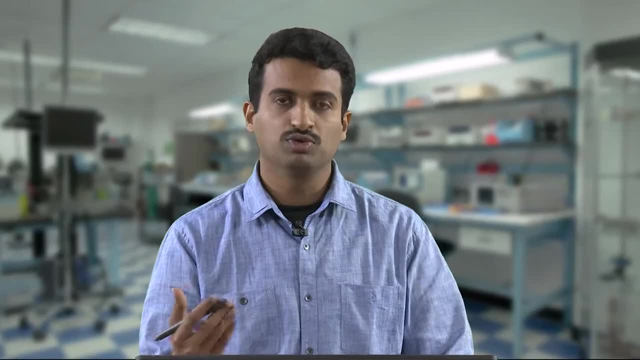 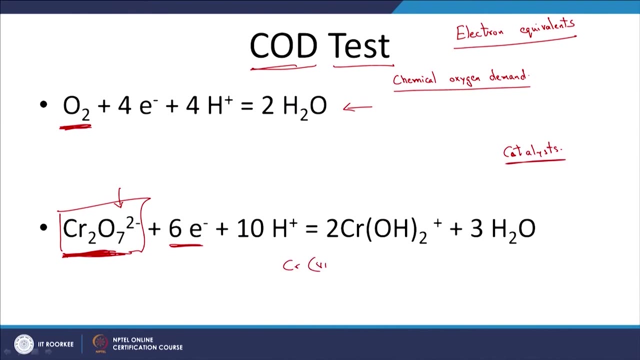 reaction that you see. So how do you go about your COD test? you either measure the decrease in the Cr2O7 2- like this: the oxidation state is 6. you either measure the decrease in chromium 6 or measure the increase in this particular form, chromium 6.. 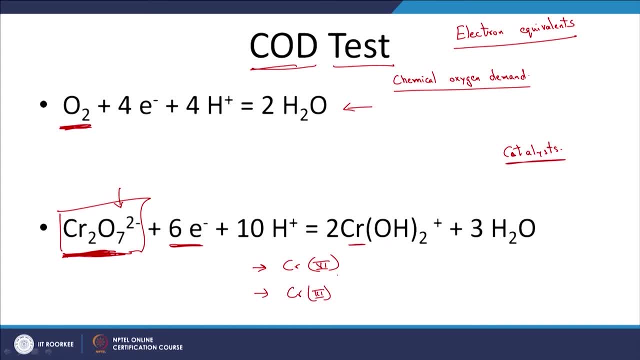 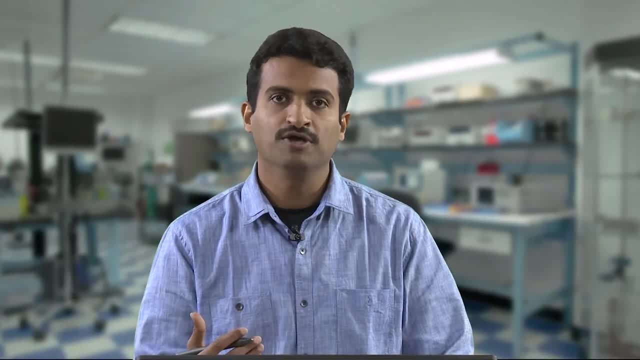 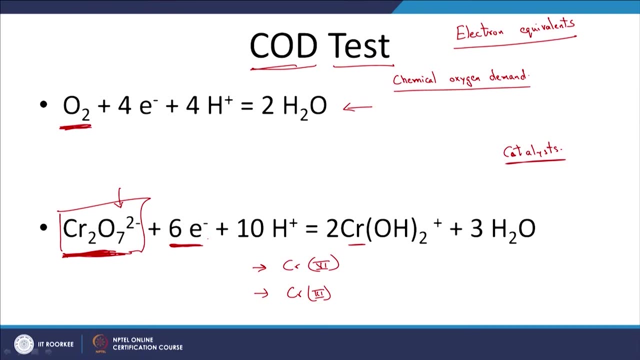 Chromium 3, the oxidation state chromium 3. so by calculating the loss of this particular Cr2O7 2- or chromium in its oxidation state 6, you can calculate the number of electrons that this particular solution would require. but to me it makes no sense to calculate the 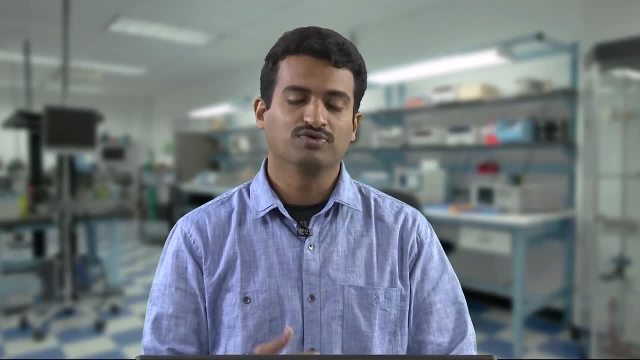 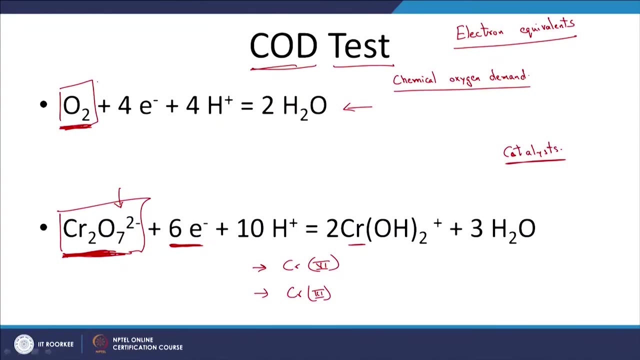 number of electrons, for example, a particular solution can donate. But I want to be able to understand what happens in the natural system, and that means the amount of oxygen, What it can consume. so here the concept of electron equivalence comes into picture, as in: you see that for 1 mole of what do we say oxygen it has, it can consume 4 electrons or 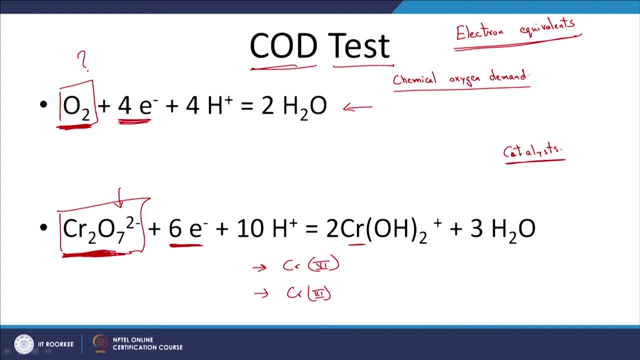 it can accept 4 electrons, But here, as you see, for 1 mole- here I am going to write that out- for 1 mole of O2, I have 4 electrons, or 4 moles of electrons, Yes, Being accepted, but in this case for 1 mole of chromium, 6, so Cr2, 6 electrons for just. 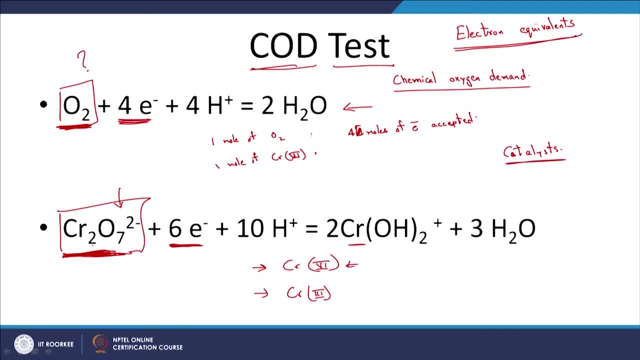 one Cr in its oxidation state of 6. chromium oxidation state 6. I will have 3 moles, or it can accept 3 moles of electrons. Yes, Yes Again. and now I want to be able to use this particular information about the amount of 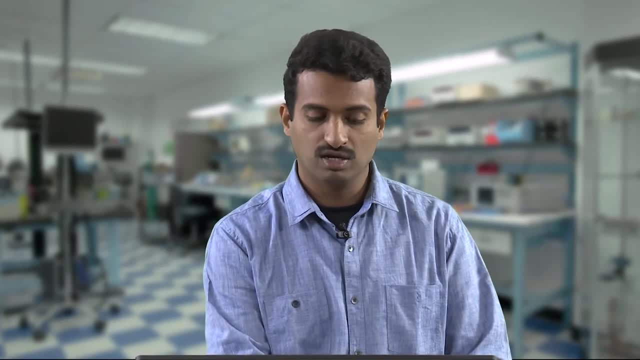 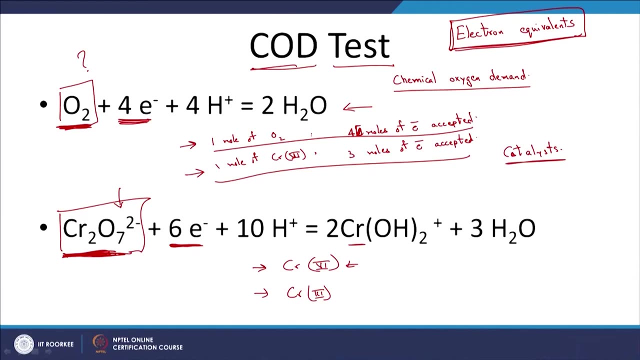 chromium 6 that is consumed to be able to come up with equivalent amount of oxygen that would have been consumed. So, obviously, what do I need to look at? I need to look at the electron equivalence. So, from that aspect, obviously, how can I go about this? I can say that for 3 moles. 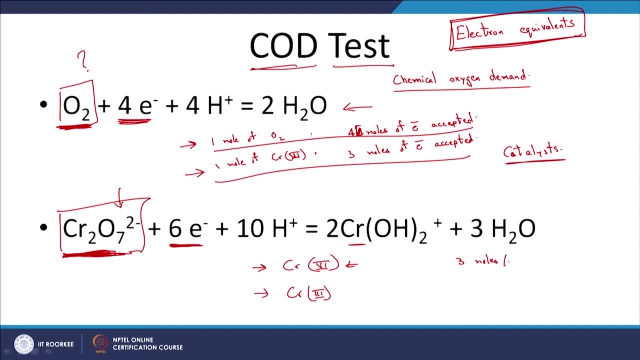 Yes, For 3 moles per litre of oxygen, 4 moles per litre of chromium, 6 would be the relevant equivalents. Yes, So again you want to balance the number of electrons. So obviously here: what is the electron equivalent? here 1 third of mole of oxygen would lead. 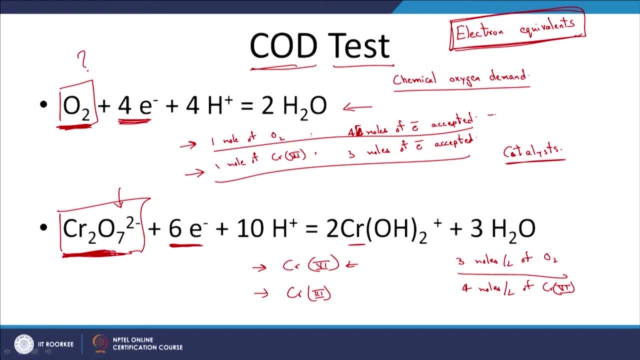 to accepting 1 mole of or 1 fourth. pardon me, So what does this mean? Yes, So 1 fourth moles of O2 would mean 1 mole of electrons being accepted and the case of chromium 6, 1 third of moles of chromium 6 would lead to acceptance of, or can accept. 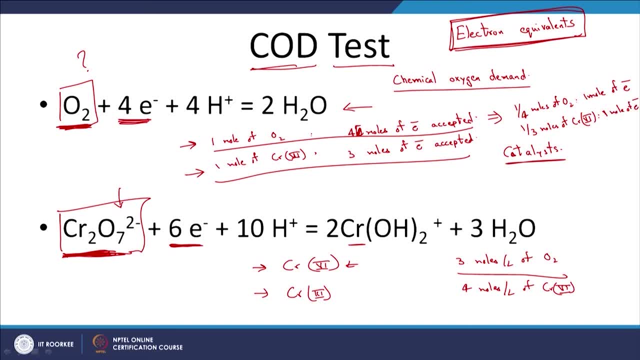 1 mole of electron, the electron equivalents. here we express them in terms of electron equivalents. So again from this particular information we know that 3 moles per litre of oxygen would be equivalent to 4 moles per litre of chromium 6.. So that is what we have here. 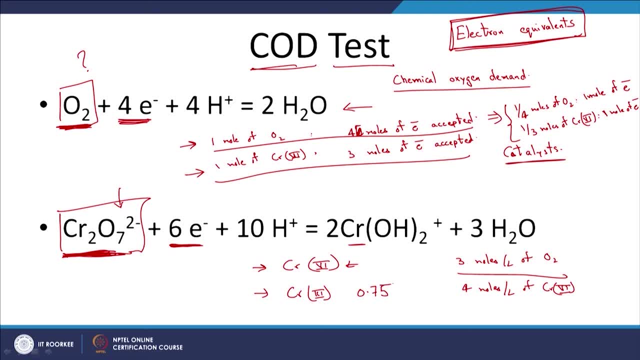 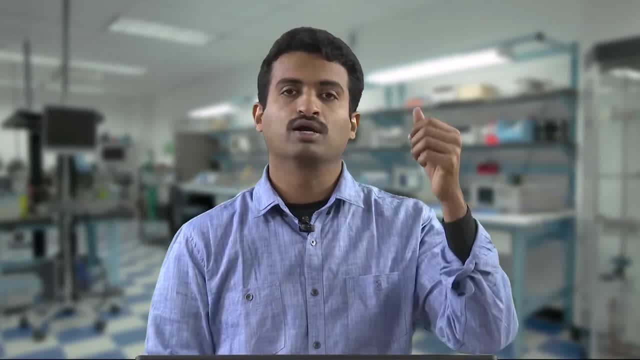 And so obviously you say you have a factor of 0.75. I guess, And this is what you would use in your CO2 test to be able to come if your chemical oxygen demand, as in you are titrating and then, or I guess, using the spectro photon meter, measuring. 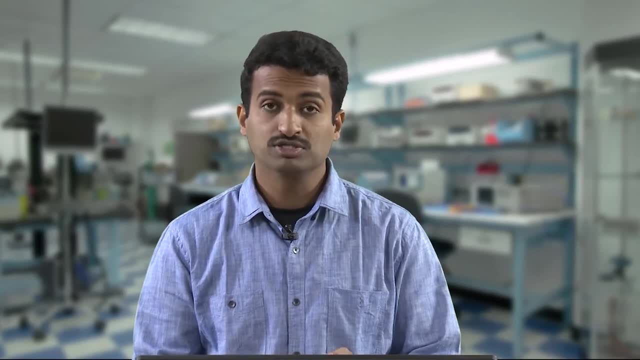 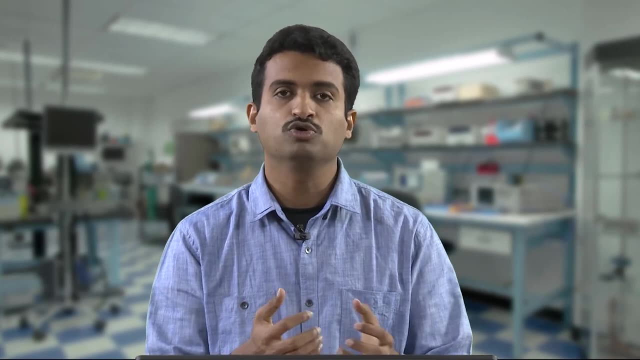 the amount of chromium 6 that is being consumed. So by using this particular factor, Yes, going to come up with an estimation- not estimation, calculation- of how much oxygen is going to be consumed and that is going to be equal to the COD or chemical oxygen demand. 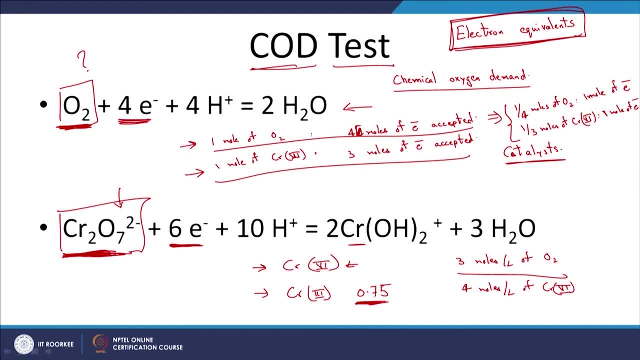 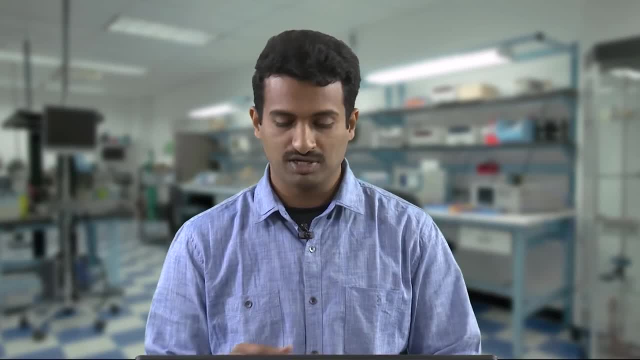 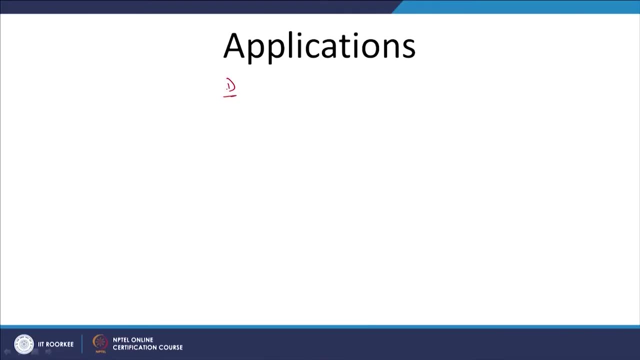 That is your particular factor, and where do we look at, or what do we look at, the electron equivalence. Now let us look at, or start discussing a few of the applications. We are going to look at a few applications here, and let us look at redox reactions, that. 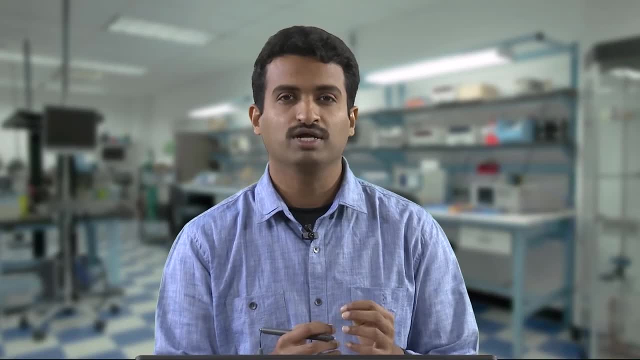 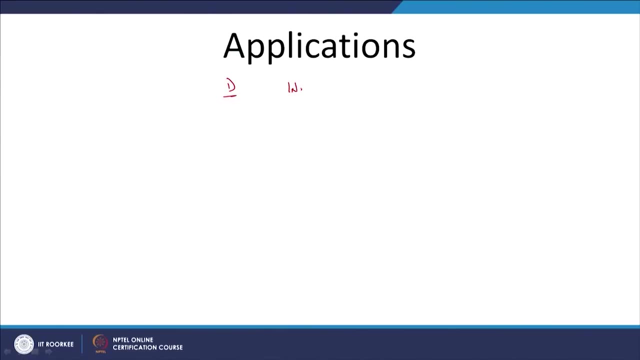 you would usually or commonly come across. One example that we looked at was in our waste water treatment plants or sewage treatment plants, You have your waste or your organic form, your organics, and now let us try to understand these in terms of the terms that we have looked at thus far. 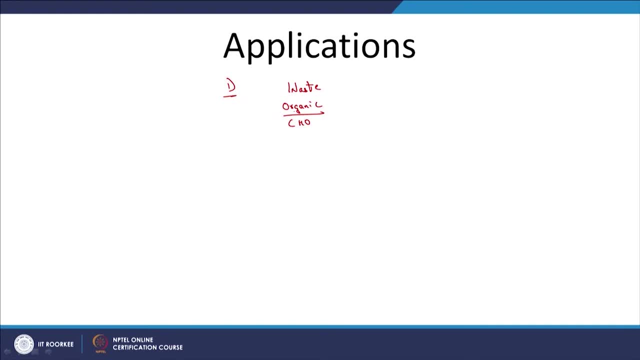 Organic compounds, usually C, H and O. Usually they are reduced forms. They are reduced forms. and now we also have oxygen, or we add oxygen, we aerate the relevant waste. and what is the process? why is it? you are trying to add oxygen, which is your electron. 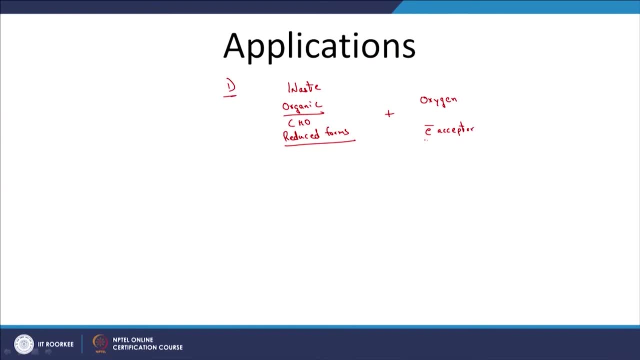 acceptor. Oxygen is an oxidizing agent and it acts as an electron acceptor and thus your organic, which is in the reduced form, will act as a Electron donor. Now you have the relevant building blocks- if I can say that- for your redox reaction. 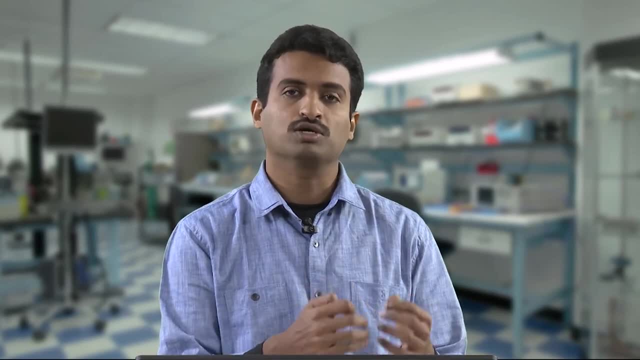 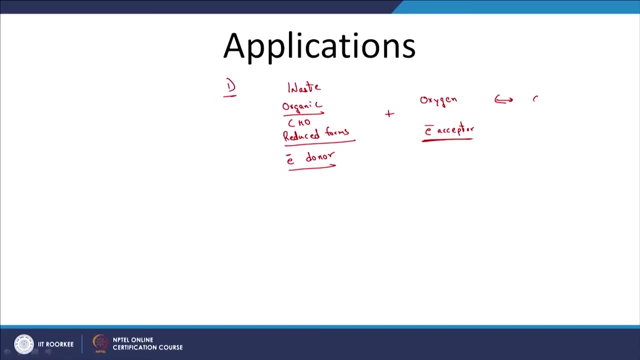 that the electron acceptor, or presence of an electron acceptor, which is the oxygen that you are putting into the waste and your waste itself is the electron donor. This can, if you look at complete mineralization, transform to CO2 and H2O. CO2 is the oxidized 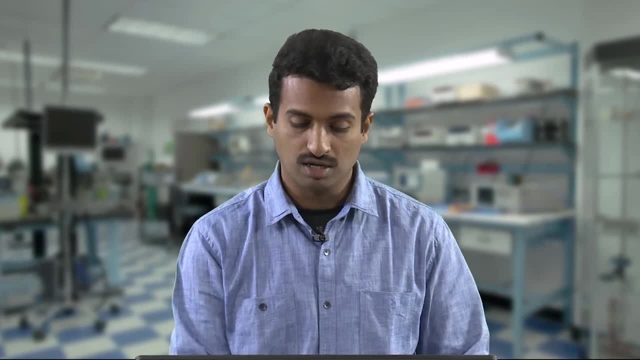 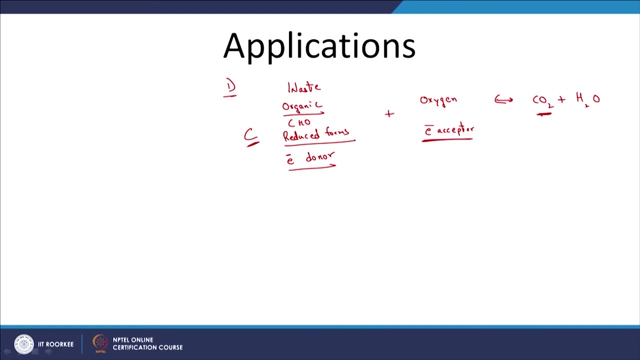 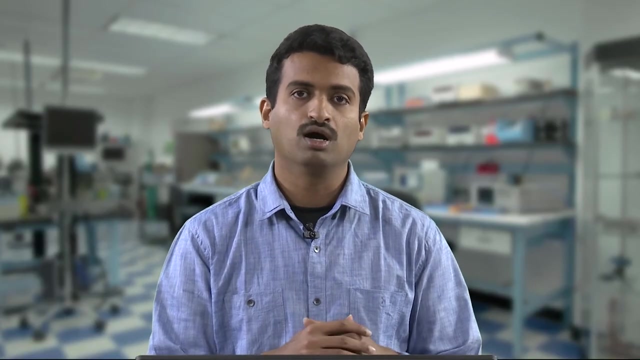 form here that you are looking at Here, C is in its Relatively reduced form, and C here is in its more oxidized form. What is happening to this particular carbon C? as in carbon, it is being oxidized by the relevant oxygen, but in nature, though, this does not take place at the relevant rates. 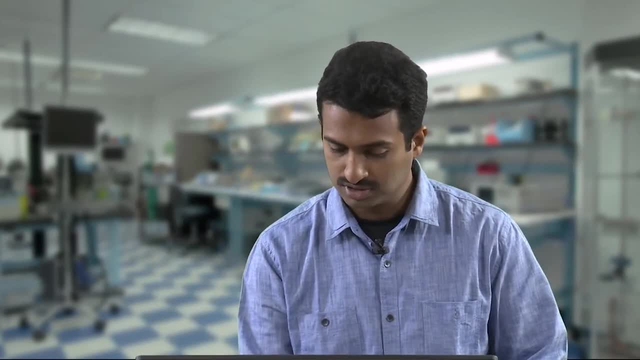 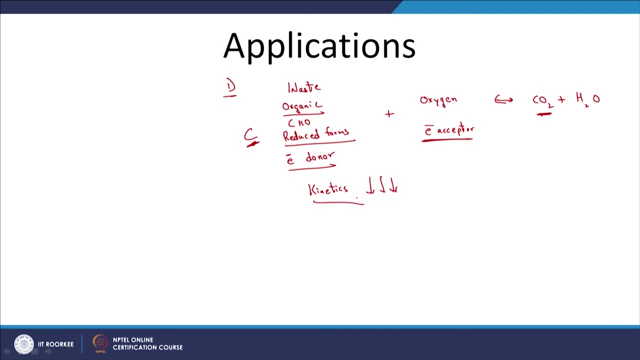 or it is not fast enough. and why is that? as we discussed, the kinetics are relatively slow. What are you doing to fast? in this process, You are going to add your seed And more or less the microorganisms. and what is the role of these microorganisms? they produce 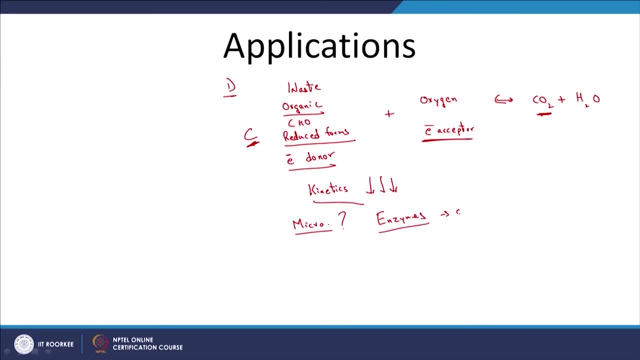 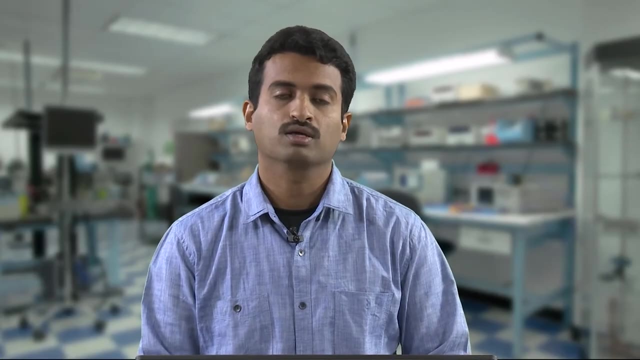 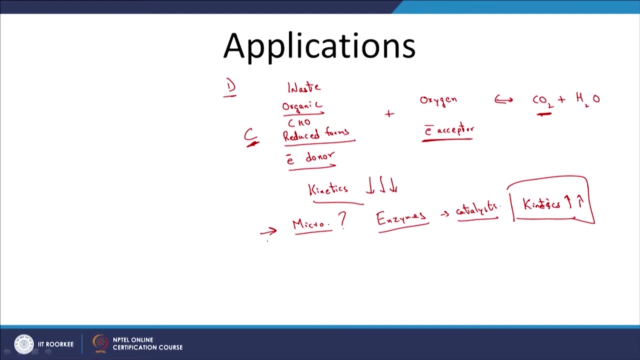 the enzymes, which then act as catalysts, thus increasing the kinetics of this particular process. so that is what you are more or less leading to, and again, keep in mind that why do these microorganisms obviously want to take part in this particular redox reaction? Well, they need to gain some particular benefit to. in general, energy is released from this. 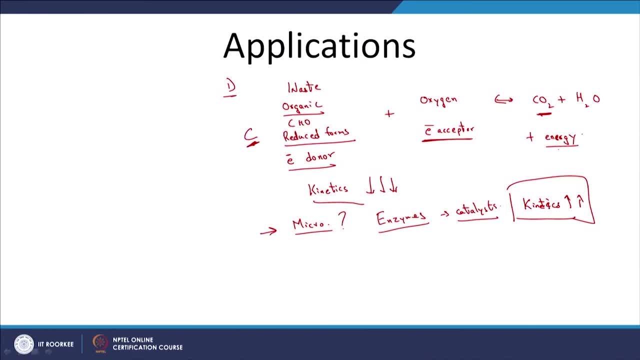 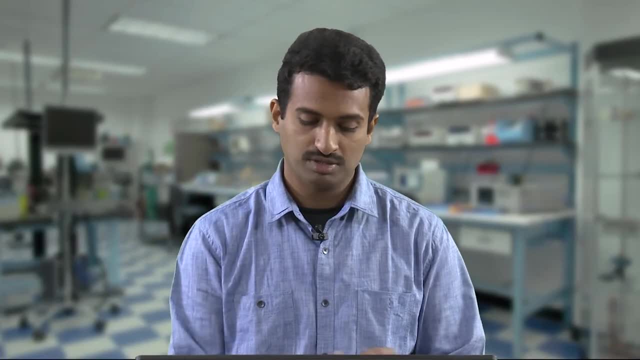 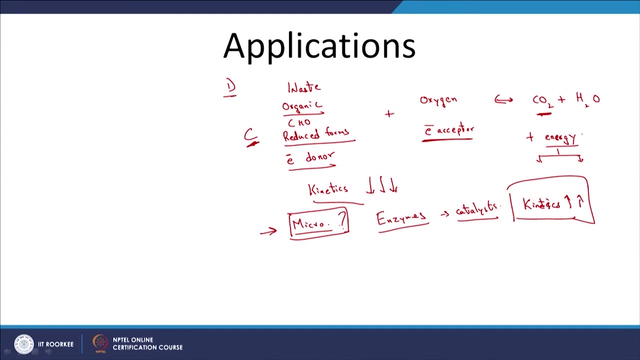 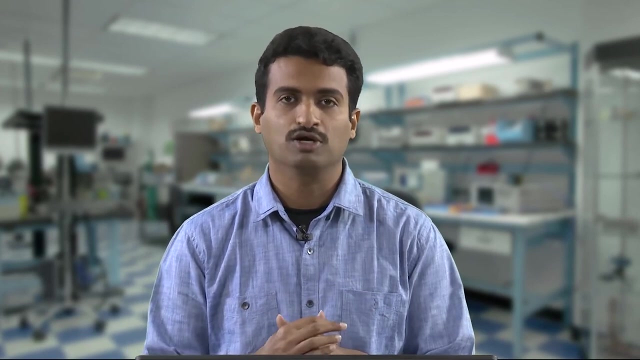 particular redox reactions and this particular energy is used either for cell synthesis, growth or such. that is the reason why microorganisms would want to degrade your particular waste. When we say degrade, we are obviously talking about microorganisms trying to extract this energy Through this particular redox process. so that is obvious example that people at least look. 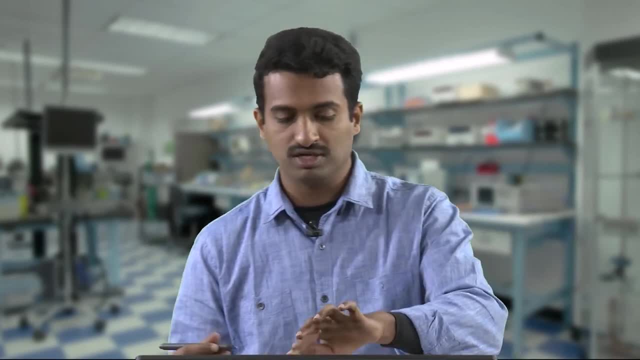 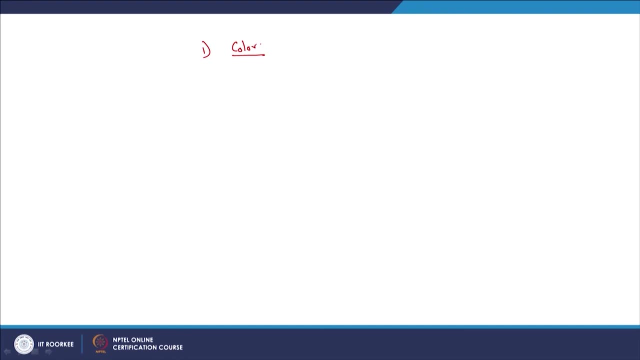 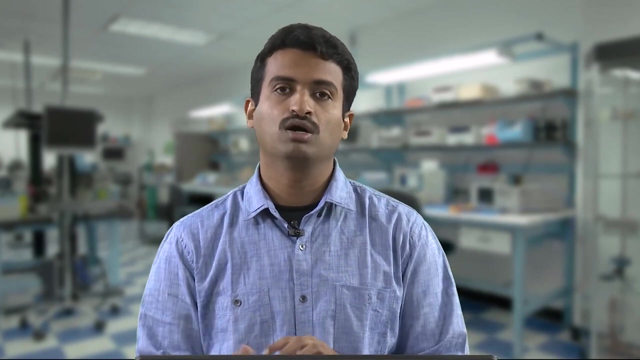 at or can look at, but there are obviously many more applications. so people talk about removing color, and what do you look at? again, these are redox process based on adding reducing agents, or, if you are looking at dying industries, color and rivers or surface waters, that is. 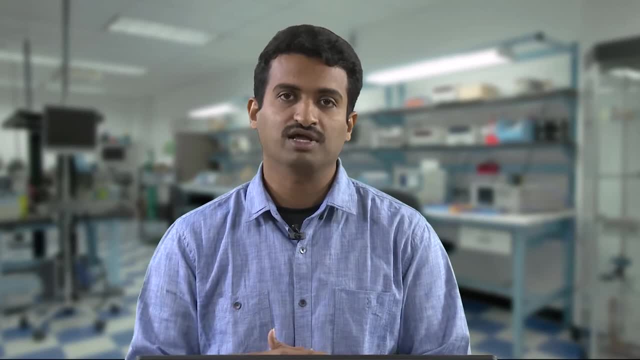 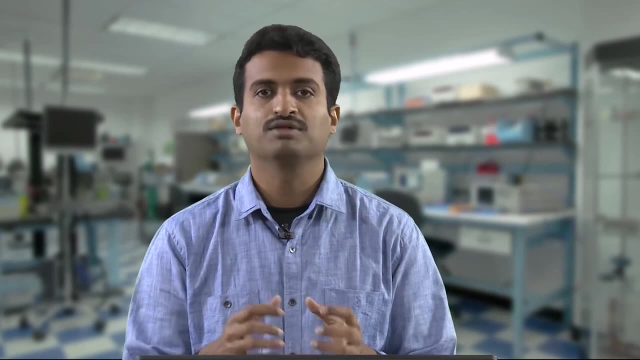 a different aspect Again, color from your dying industry. that is again a different aspect. but more or less, what do you add? you need an oxidizing agent, and oxidizing agent, as in it, is an electron acceptor and that again, when we are talking about color removal, we are in general again. 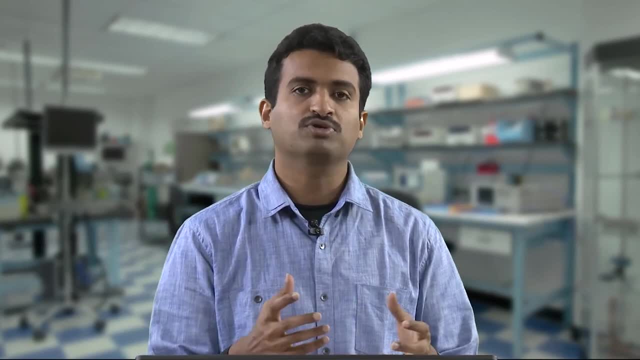 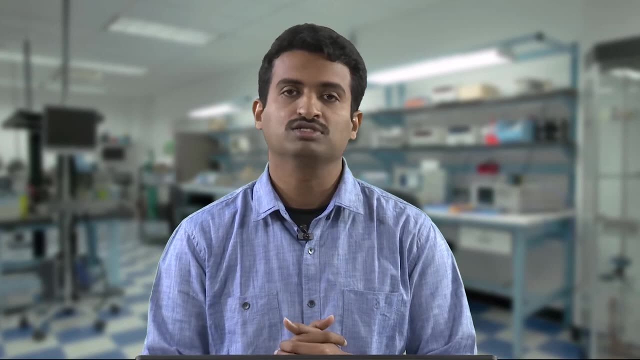 obviously talking about your redox process. So again, when people talk about taste, there is certain compound that is leading to this particular taste or such and you can add the relevant oxidizing agent or such to be able to remove this or oxidize this particular contaminant. 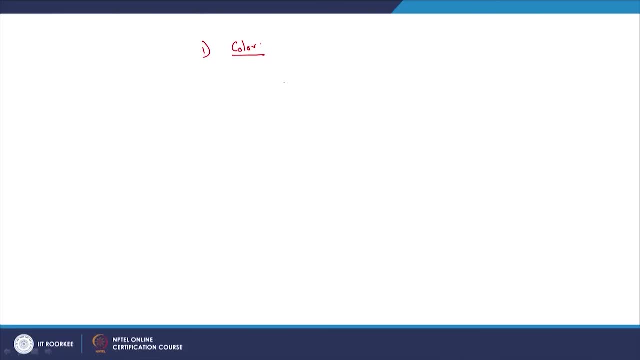 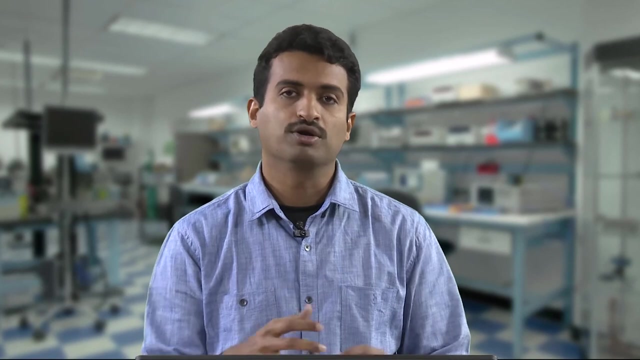 So in this context again people come across advanced oxidation process. so advanced oxidation process- and obviously we are calling this advanced oxidation process because we usually lead to, or these particular AOPs lead to, or there are different kinds of AOPs I should have listed. 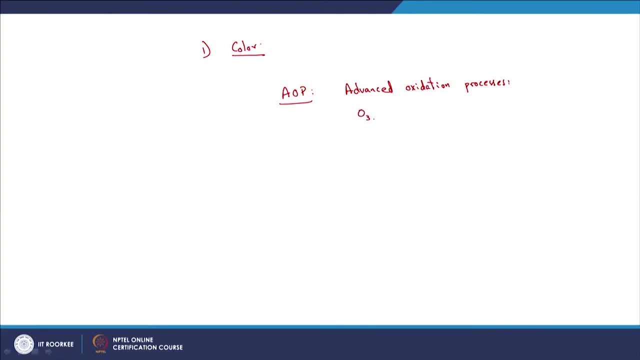 First, just ozone. if you vary the pH depending on the change in pH and ozone with respect to UV or H2O2, or in conjunction all three of them, and UV, H2O2 process, UV as an ultraviolet and H2O2, and phenton's reagents too, Fe2 plus and H2O2.. 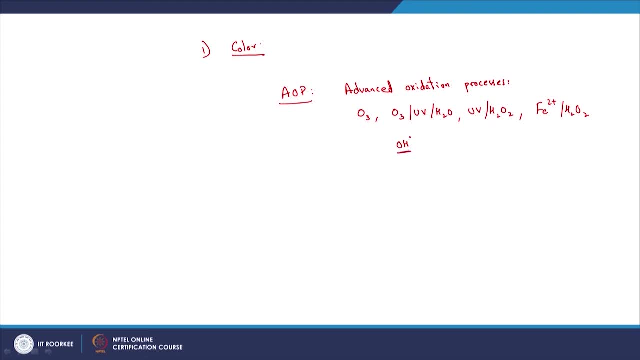 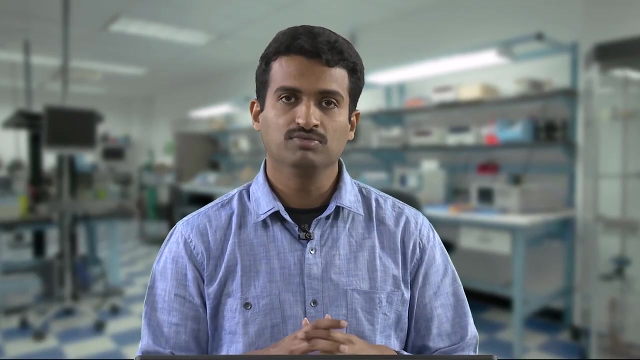 This can lead to formation of your radicals, more specifically, your hydroxyl radical. and what is this radical? It is an unpaired. it has an unpaired electron. So this hydroxyl radical has an unpaired electron, so it is remarkably unstable. so it wants to. 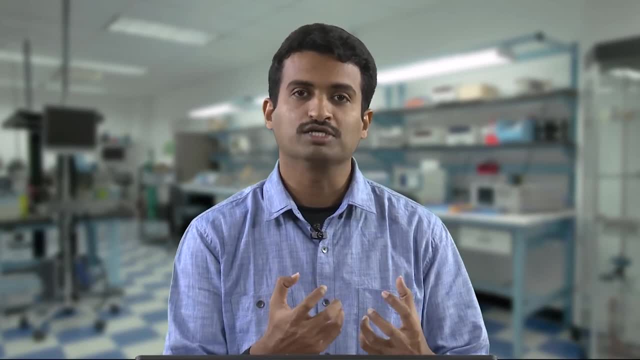 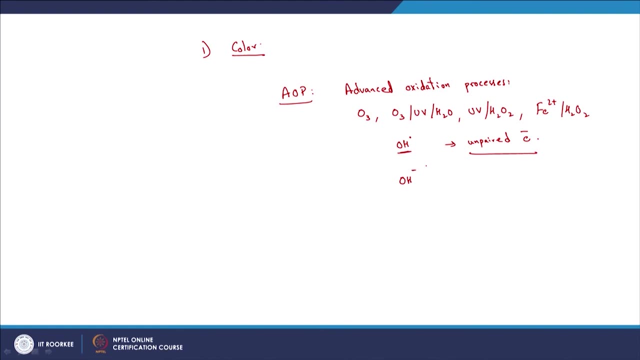 what do we say? it tends to try very hard, if I can use layman's terms, to accept electrons and go to its more stable state, which is going to be OH- so thus, OH radical, this is a radical and in this context, the radical is stable. 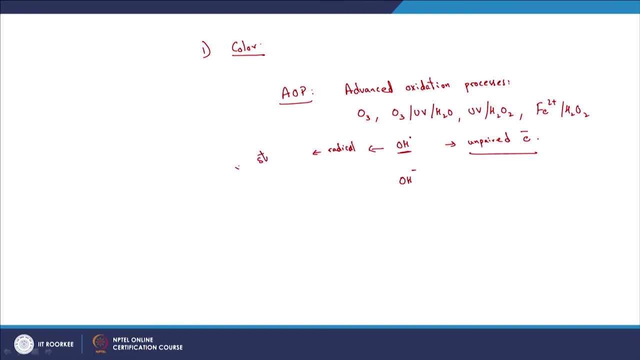 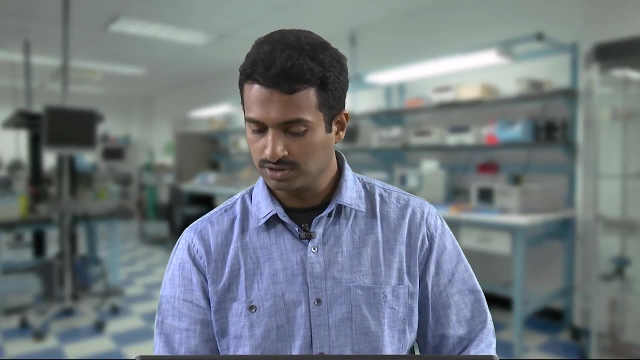 Let us say, is a stable radical. So this is a stable radical. It is a very strong, or very strong, very strong oxidizing agent, Similar to these hydroxyl radicals. depending on the relevant- what do we say? mechanism you look at, you can also produce these reducing radicals, which is the hydrogen radical, and 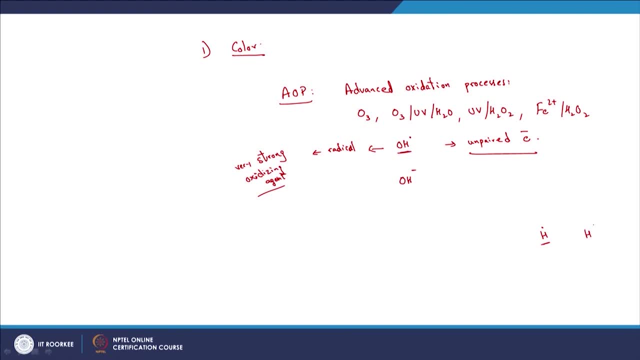 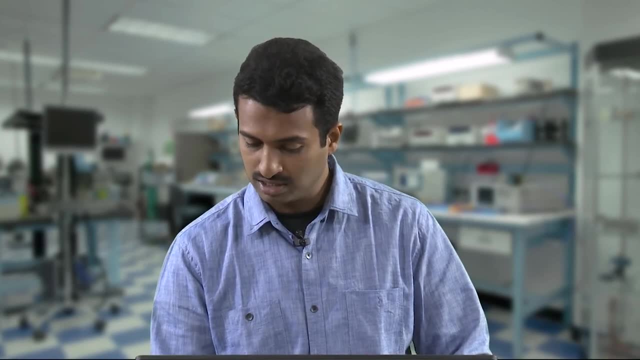 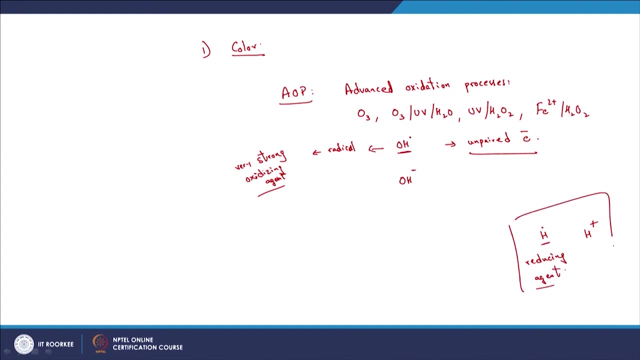 obviously, you know, hydrogen radical would want to go to its more stable state, which is H plus, as in, it wants to release or donate its electron, Which the hydrogen radical will act as a very strong reducing agent. this is a different aspect. I want to highlight that because here we are talking about the oxidizing agent, which 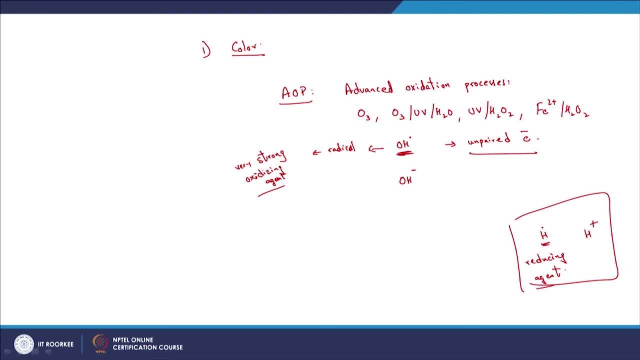 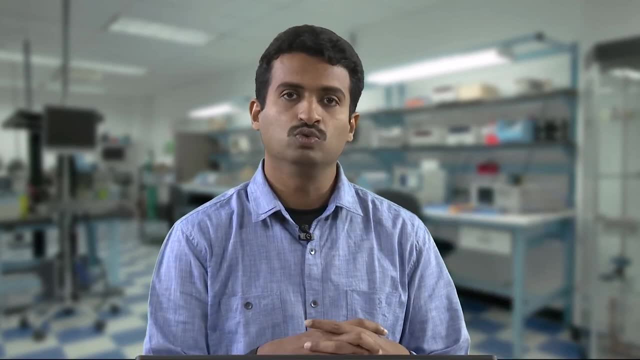 is the hydroxyl radical here and the hydrogen radical can also be formed in different what do we say process? So in these AOPs, have what do we say applications with respect to situations when your particular ways are relatively non biodegradable If you are using biological process? 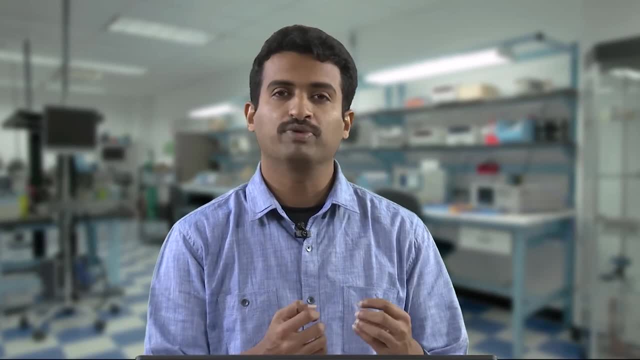 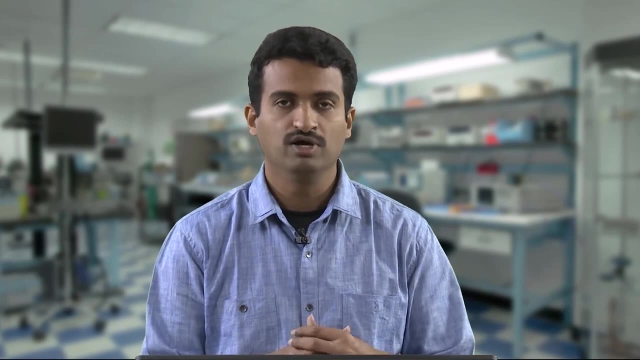 So this is a very strong reducing agent. So this is a very strong reducing agent. If you are using a non biodegradable process and your particular ways are relatively more biodegradable, then the relevant efficiency of the process is, or would, be good enough. 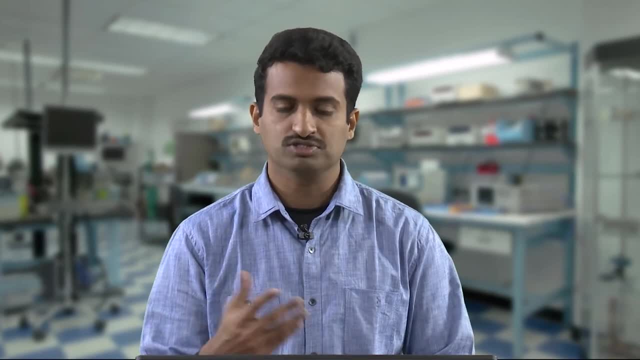 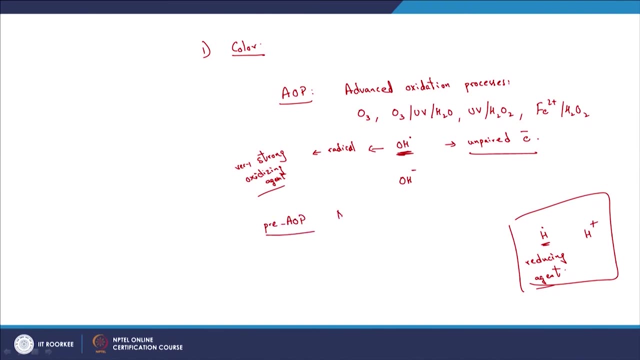 But if it is not, and if you want to increase the efficiency of the process, one way would be to have pre-AOP. then your non biodegradable wastes- non biodegradable wastes- will be transformed after application of these advanced oxidation process into biodegradable wastes. 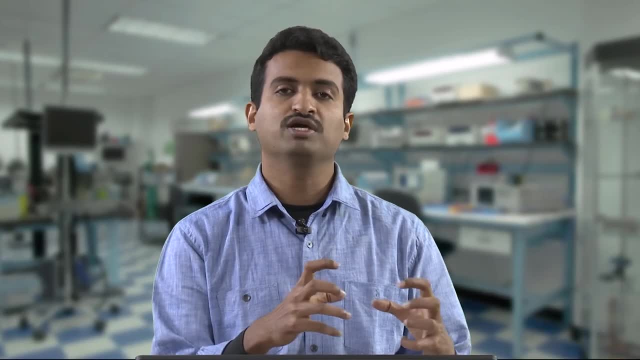 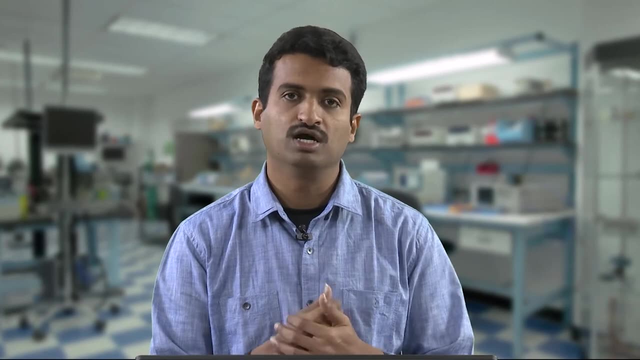 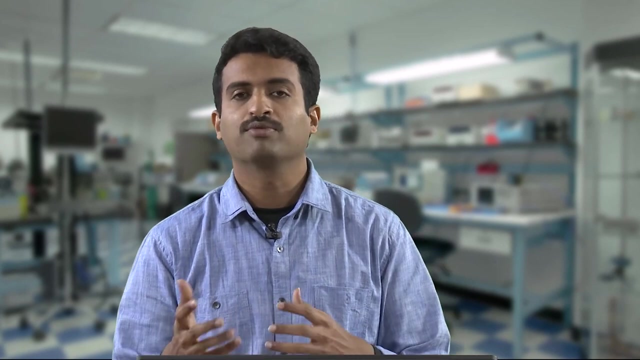 You have a non-biodegradable waste for which your particular ASP or SBR is not that efficient, or the kinetics is taking way too much or way too long, or kinetics is relatively slow, and also even your final product is not up to your standard. What can you do? You can either just use advanced oxidation process, but there might be practical limitations with respect to cost involved. With relevant doses of AOP, you can transform this non-biodegradable waste into biodegradable waste and then use your biological process to degrade or mineralize these particular. 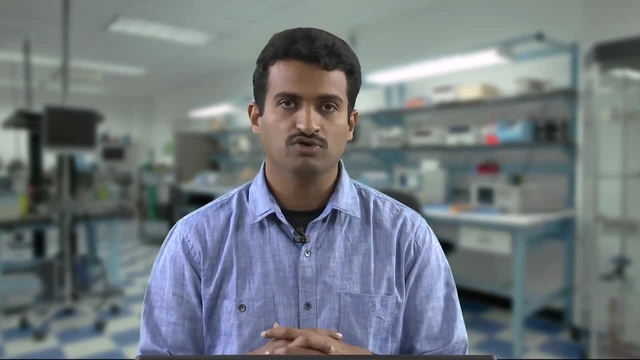 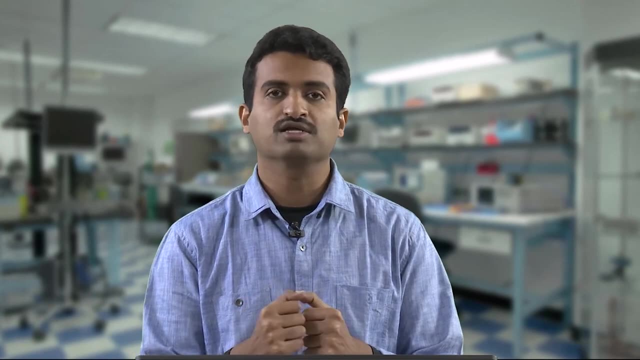 biodegradable waste. In effect, you are increasing the efficiency of your process. There are many more applications. We will look at a few more in the next session and then we will move on to first understanding this concept of oxidation state. We have oxidation states, oxidation numbers, 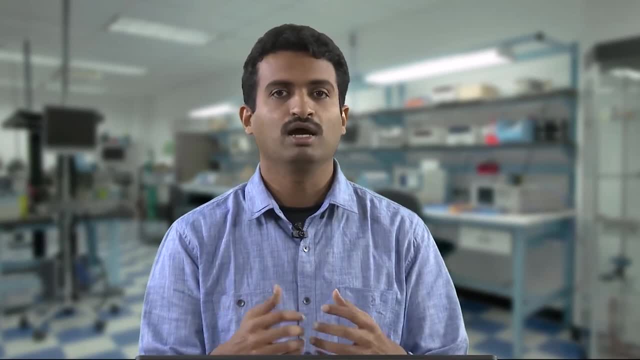 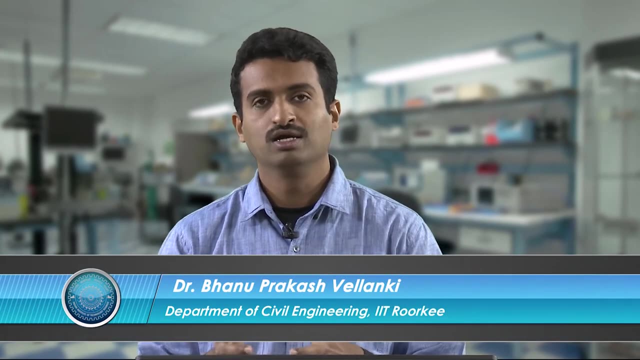 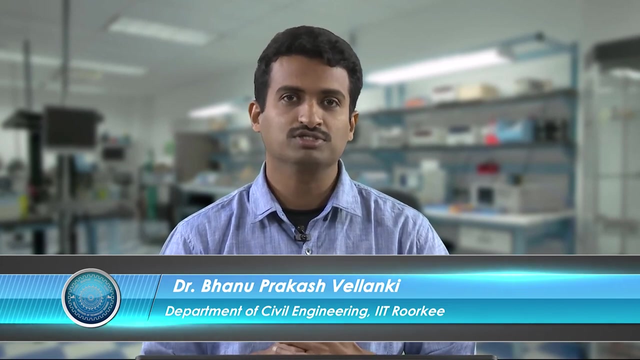 What is this? How do we calculate that? It is relatively simple, but maybe people have looked at it in great detail. But this is at the crux of what we are going to look at in this particular set of sessions. We are going to look at that in greater detail, and with that I will end today's session.